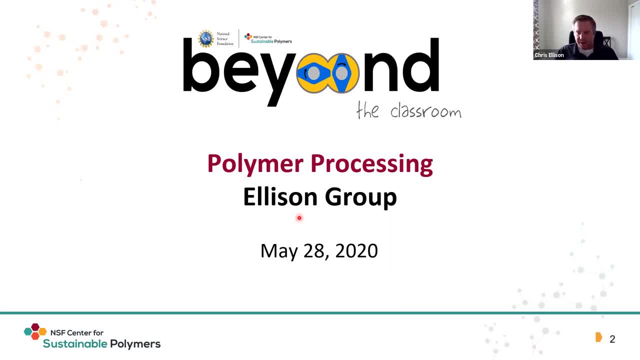 processing. I want to thank a lot of people from the Ellison group that have helped put this together. You'll see their names and their pictures as we go through and you'll hear from some of them as well. I want to give special thanks to Boran Zhao and John Beamer, who helped. 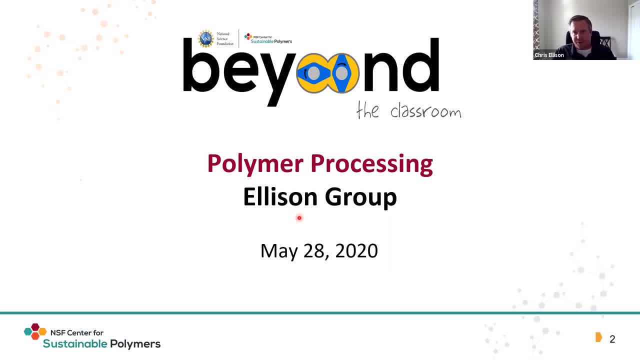 make the beyond logo with the two kneading blocks. You'll see reports of the two kneading blocks replacing the O. These are kneading blocks that you'd see as part of a screw and a twin screw extruder. that's co-rotating, So it's relevant to the topic today. Also want to 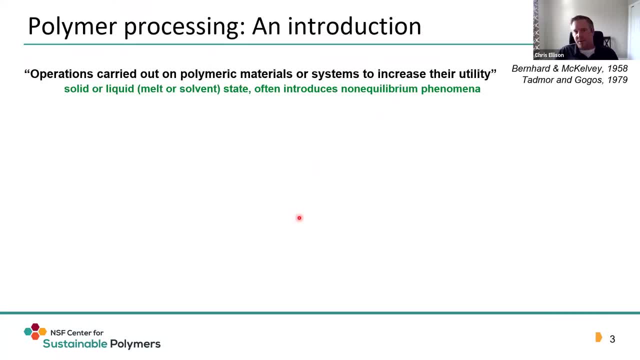 thank Chris Micosco who helped give feedback on some early versions of this talk. So just to start, I want to lay a little bit of the foundation of polymer processing, introducing it, but also talking a little bit about how it's intertwined with material properties. Of course, processing 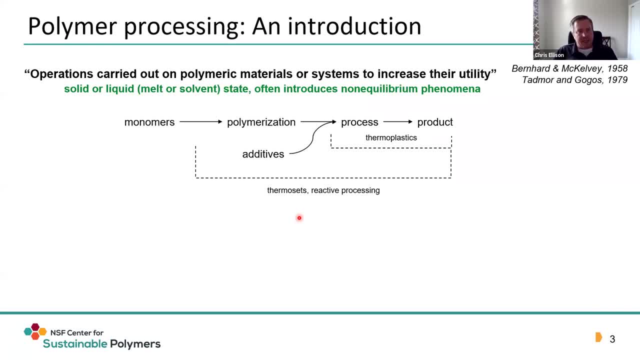 polymers really increases their utility substantially. Processing can take place in the solid or liquid state, and liquid can be produced by way of heating to make a melt or by adding a solvent. But as you'll see in a moment, this often introduces non-equilibrium phenomena. Sometimes we take advantage of it to produce. 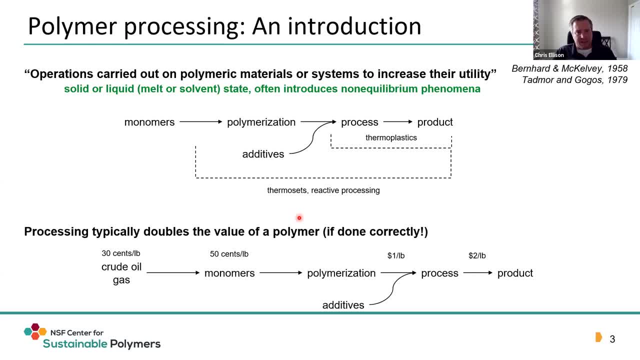 unique properties and other times we'd like to reduce it to prevent other phenomena. Polymers can be processed in a number of different forms. The next image below shows thermoplastics, where you may heat a series of pellets, run it through a process to make a product. but you can also 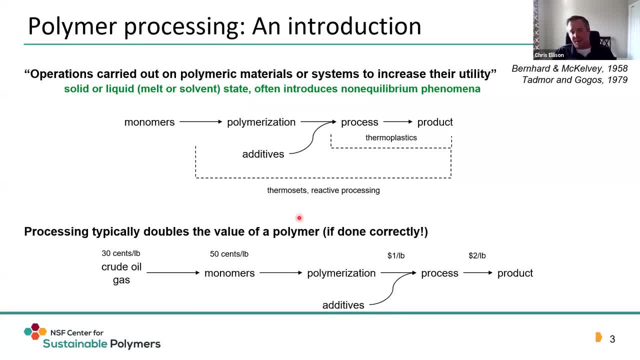 process thermosets by way of reactive processes. For example, if you wanted to make epoxy composites, you might take reactive monomers and process them in a carbon fiber woven mat. Processing typically doubles the value of the polymer, if done correctly, and so below I'm just sort of showing the flow of 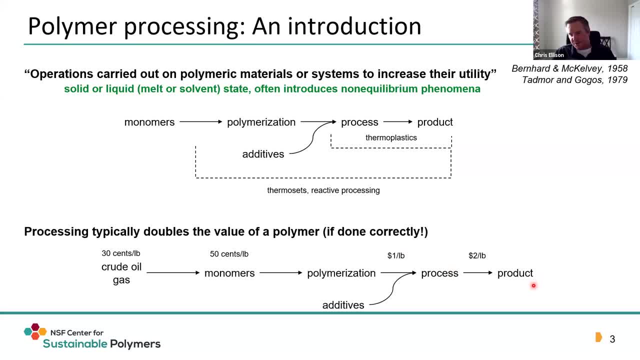 from cradle to grave, so to speak, or crude oil and gas, entering at the beginning, Of course, in the Center for Sustainable Polymers we hope that that would be biomass or sustainable materials. And then finishing at product, and you can see, it goes from one dollar a pound. 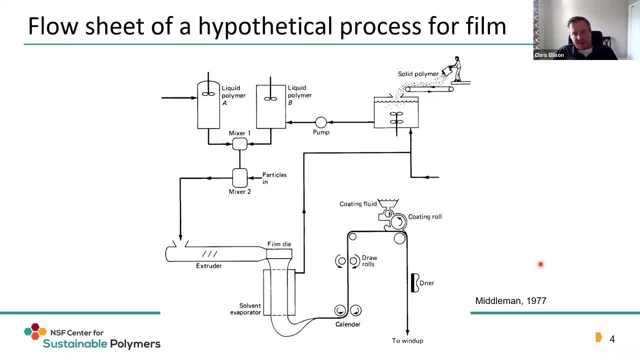 to two dollars a pound by way of the process. The process can be pretty complicated. Here I'm just showing a flow sheet of an hypothetical process for film, and really the only takeaway I'd like you to have here is that the process is more complicated than sort of the. 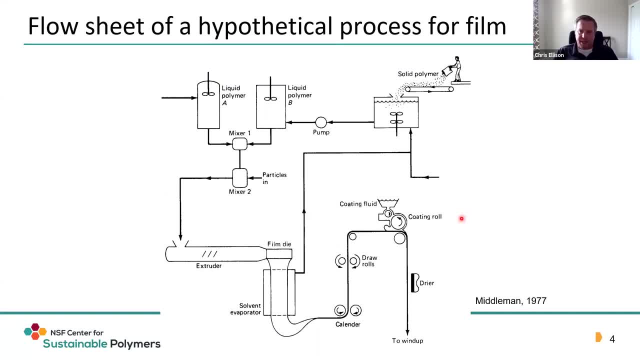 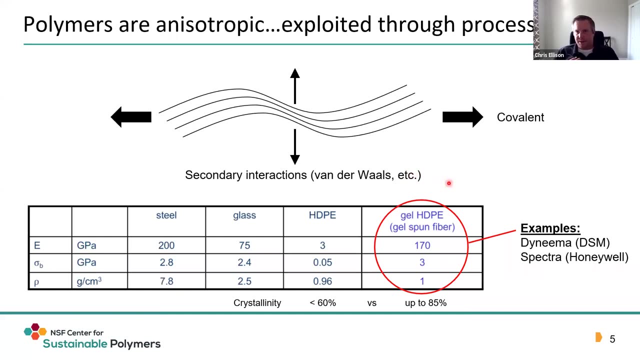 single units that we'll show you today, and you really need to think about it in terms of all the unit operations. Here I'm showing a film process, just as as an example. Okay, next slide. Polymers are anisotropic, and so this, this is typically exploited through. 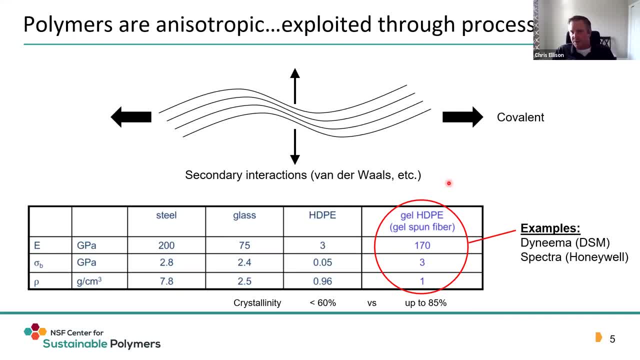 processing. because they're long chain molecules and have covalent bonds, They can be aligned in the flow and that alignment in the flow can and can impart unique properties that can compete with more conventional materials. In the table below I'm showing you the modulus, the strain at break and the density for steel glass. 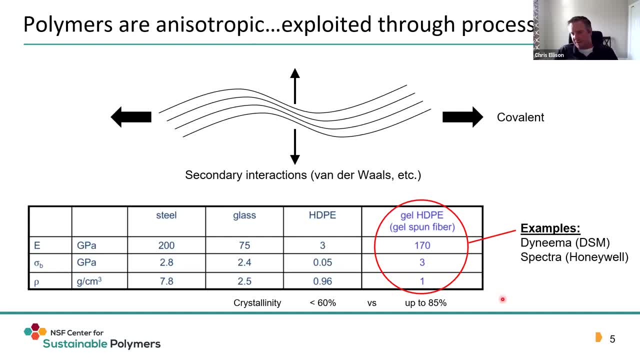 HDPE and gel spun HDPE, which is a fiber spinning process, And you can see that HDPE that's just maybe ordinarily processed by, let's say, molding, The properties are not that competitive with steel and glass in terms of modulus, strain at break, etc. However, if you process it by 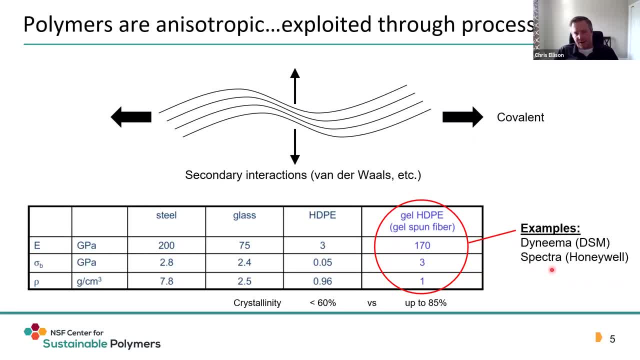 gel spun fiber process, you can actually make fibers that are competitive with steel but have almost eight times lower density, And so this is a a result of alignment of polymer chains. This is sold as several different commercial products, One by DSM called Dyneema, and the other by Honeywell. 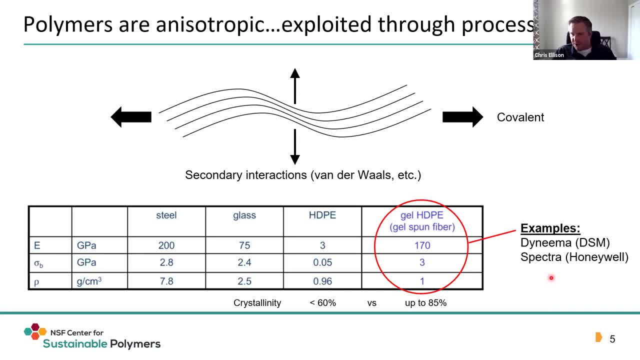 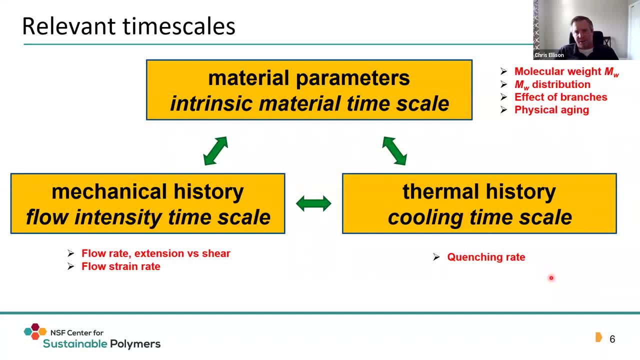 And this is a product called Spectra. So the role of the material in the process is actually quite important in defining the final properties. One of the ways you might think about how materials are intertwined with the process is to think about relevant time scales. 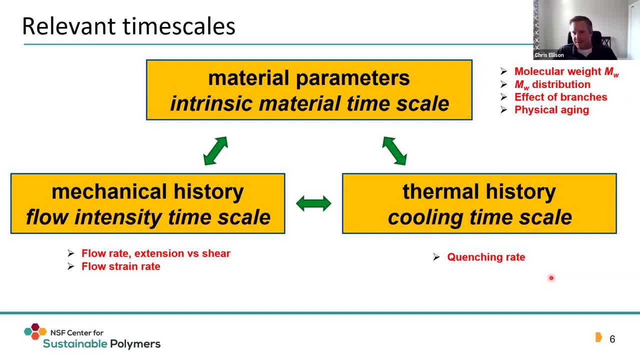 Of course materials have intrinsic material time scales. These might be related to things like the relaxation time, Could be related to the crystallization kinetics, And these are dictated by things like your weight distribution, branches, physical aging, etc. But you have to think about those material time scales and how they 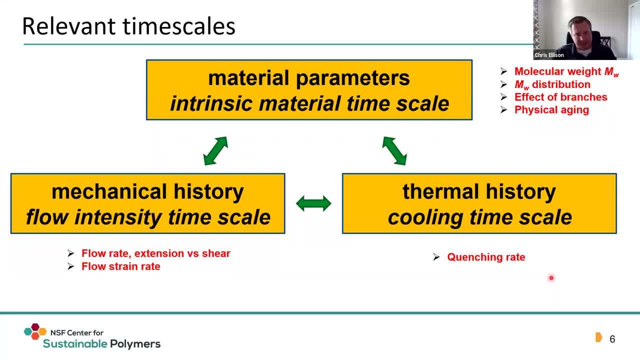 how they work with the process, which come from the mechanical history, The flow intensity, time scale, which can be different depending on the process that you're using, And then also the thermal history. Thermal history in particular is important by way of how quench rates may control internal stress. 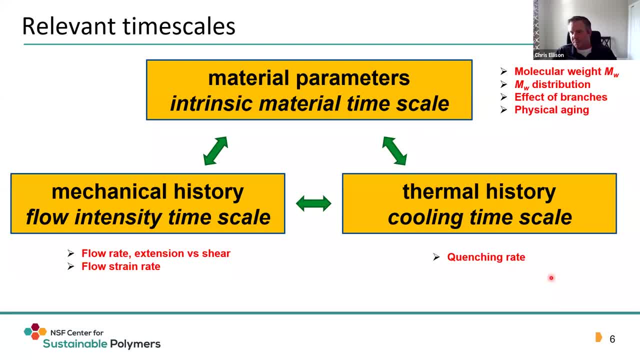 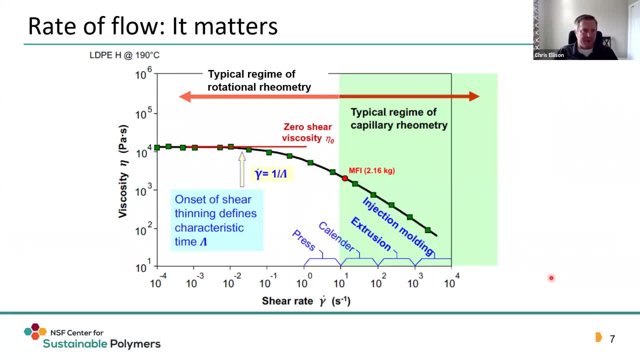 Or the stress in the system, or the crystallization kinetics and ultimately the crystal content. So these three time scales are really important, Just to show a few examples of this. I'd like to focus on the rate of flow and how it can affect the way in which a material behaves, And here I'm showing low. 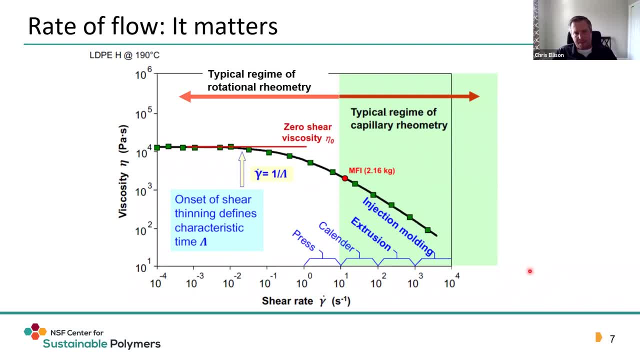 density- polyethylene, the plot of viscosity versus shear rate, And you can see that the viscosity that the material exhibits in the process can be very different than the shear rate or the characteristic shear rate of that process. So you can see injection, molding, extrusion, calendaring, pressing or molding. 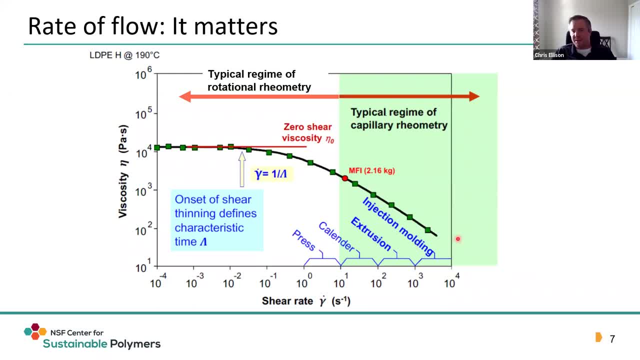 can all take on different characteristic shear rates, And this means that a given material may adopt several different viscosities in several different types of processes. I'd just like to point out that measuring the rheology or the viscosity of these systems over such a wide shear rate range, 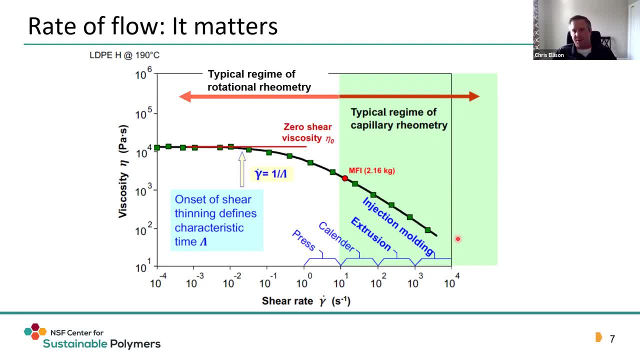 typically requires you using several different types of rheometers: Rotational rheometry at low shear rates, and then capillary rheometry at high shear rates. So rate of flow matters substantially. The type of flow is also quite important, And so here I'm showing the shear. 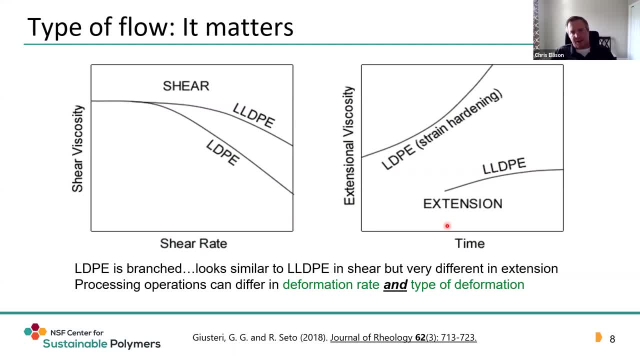 viscosity and the extensional viscosity, comparing low density polyethylene to linear low density polyethylene And you can see that the shear viscosity of those two systems look relatively similar in their contrasting response. So if you see my image here, you can see that the shear viscosity of these two systems looks relatively different. So you 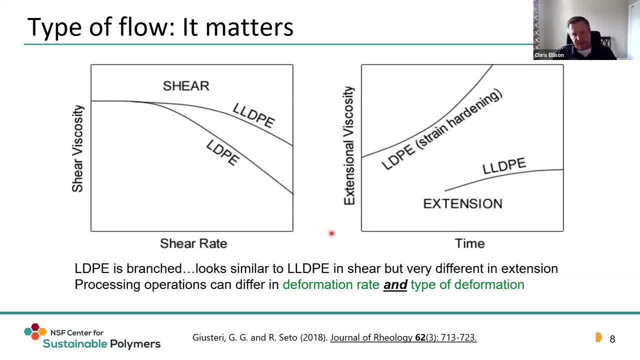 relatively similar. They both shear thin and they're not that different. However, if you look at the extensional viscosity, which is a different type of flow, the LLDPE doesn't exhibit much extensional strain hardening, while LDPE strain hardens substantially, And so the reason for this. 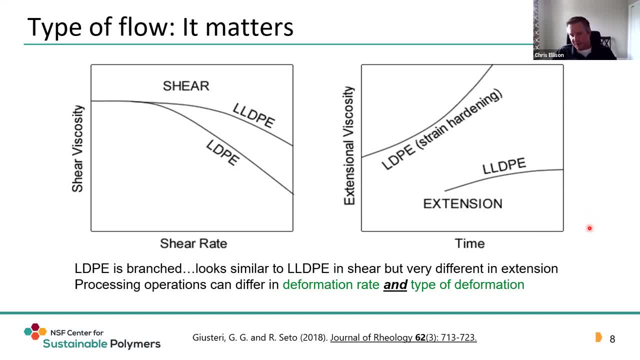 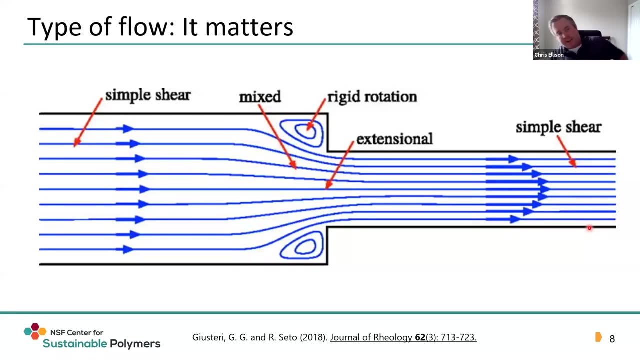 is. LLDPE is highly branched. It looks similar to LLDPE and shear, but it's very different in extension. And this all comes from two polymers that are essentially all carbon and hydrogen. So keep in mind that processing operations can differ in both deformation rate and the type of 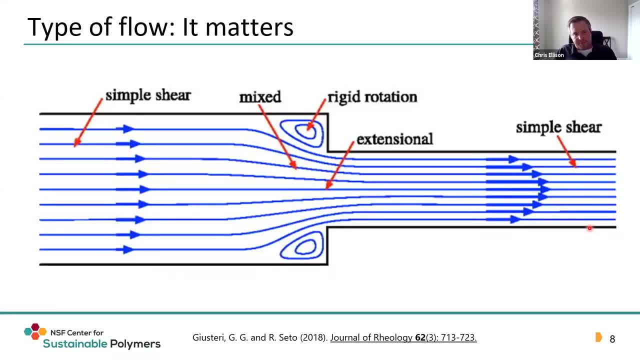 deformation. And here's an example where both the type of deformation and deformation rate differs in a single process. So it's not as If you take one process and it has one type of shear and one type of shear rate. it can actually exhibit multiple types. So this shows the streamlines of the fluid: a polymer melt. 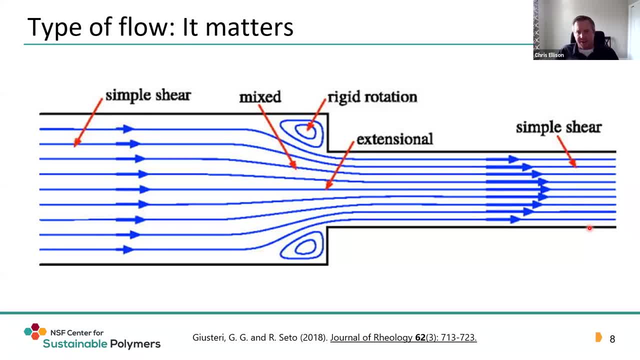 let's say, and the size of the arrows indicate the velocity of the flow, And essentially you have a large tube going to a small tube And where this contraction happens, there's a significant amount of extensional flow or mixed shear and extensional flow, Whereas at the ends of 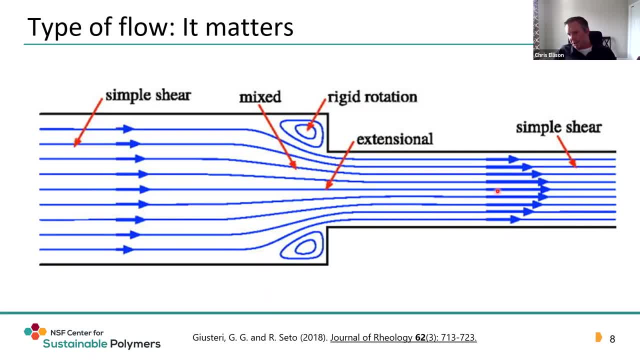 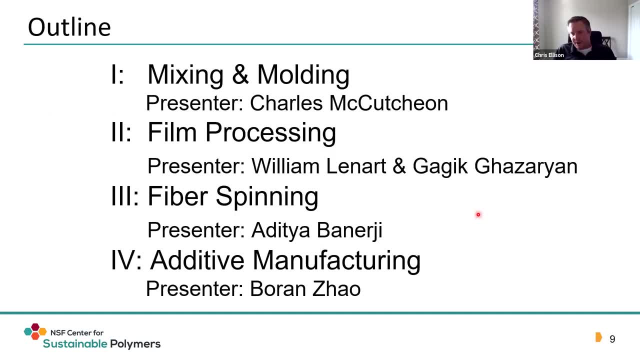 both ends of this picture, you typically just have simple shear and roughly parabolic velocity profiles, And so this is a very simple flow, but it has a very complicated type of shear rate and type of deformation. Okay, so this is the outline for our talk And I won't spend too much time on. 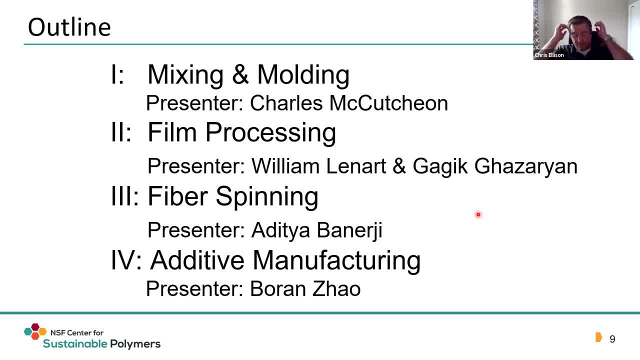 this because you're going to hear from all these presenters as how we've divided it up. One of the comments I'd like to make from here forth is that we put this talk together with quite a few details within the spirit that you may access it at later time as a starting point as you begin to think. 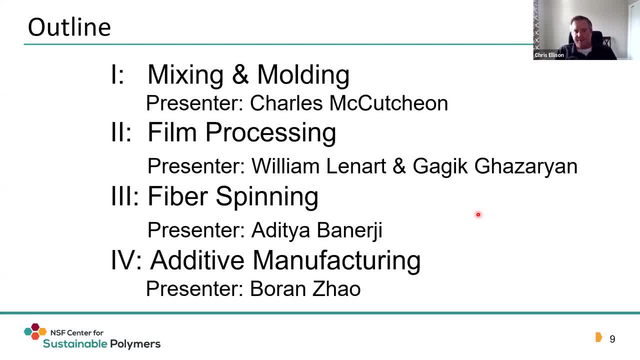 about processing, So we may not cover every single detail. This isn't how I would normally put together a technical talk, but in the spirit of you having the information to access at a later time, we decided to put it together in this manner, So I'll now turn it over to Charlie. 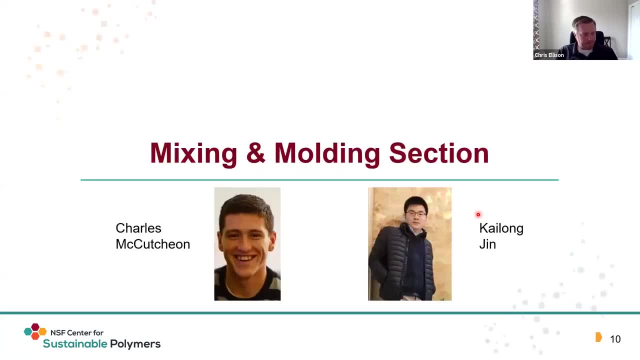 He'll cover mixing and molding. Hello, I'm Charles McCutcheon. I'll be discussing mixing and molding. I'd like to just note that if you have any questions about this section, feel free to reach out to myself or Kailong, and we'd be happy to answer them for you. 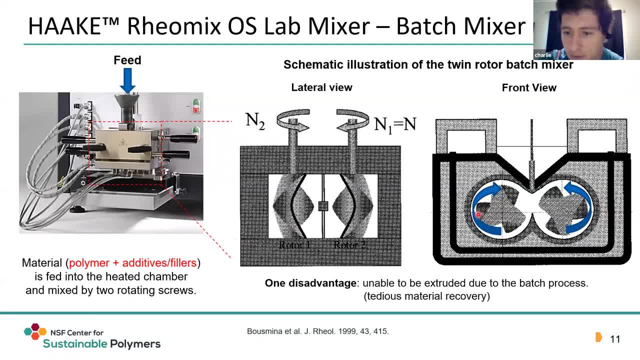 And one more thing I'd like to address at the beginning is that, for all the mixers we will discuss, they can be used to mix polymer-polymer, polymer-additive and polymer-filler type of blends. So the first mixer we'll talk about today is the Hake Rheomix Lab Mixer, which is a batch mixer. 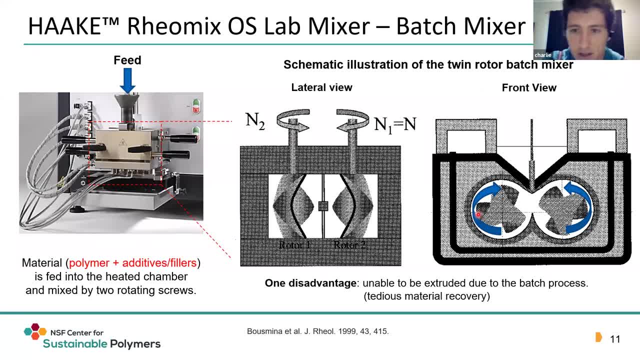 So the general process is: there's a feed so you could put in whatever type of polymer or filler you would like, and then it goes into a heated chamber where it is mixed. You could see two cross-sectional views: a lateral and a frontal view. 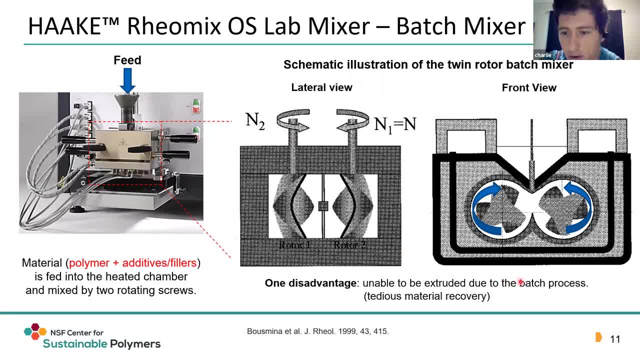 and you could see a visual of the screws. The screws are counter-rotating and you could see the mixing flows. Like I mentioned earlier, this is a batch process and therefore one disadvantage of it is the material after mixing is a little difficult to recover. 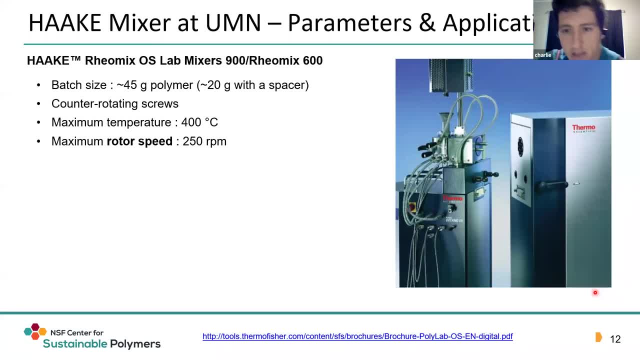 So the specific Hake mixer we have at the UMN is a Hake Rheomix OS Lab Mixer 900.. So the batch size is about 45 grams. or you can do a smaller batch size, about 20 grams, with a spacer. 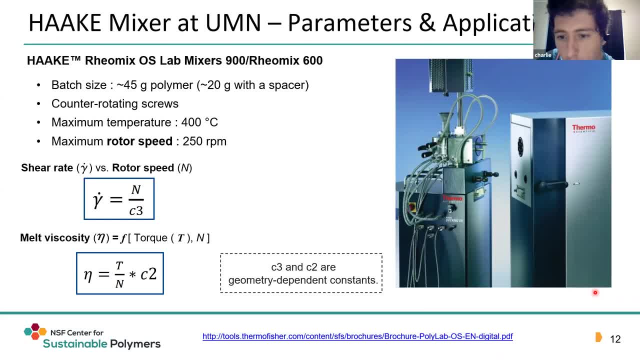 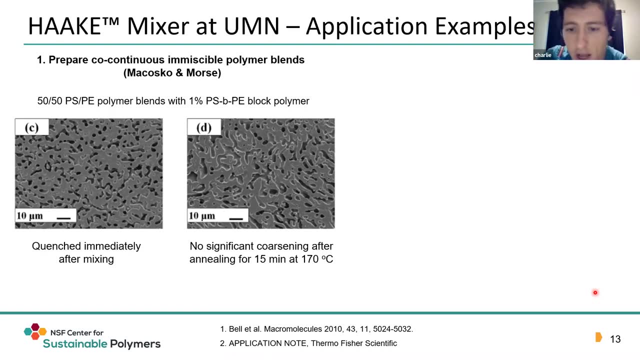 You can do in-situ measurements while mixing, Such as the shear rate, which is proportional to the rotor speed, and the melt viscosity, which can be measured from the torque and rotor speed. So an example of research that used the Hake at the U of M was done by the Macasco and Morse group. 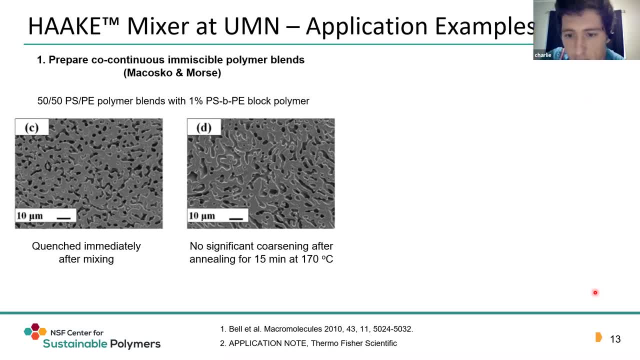 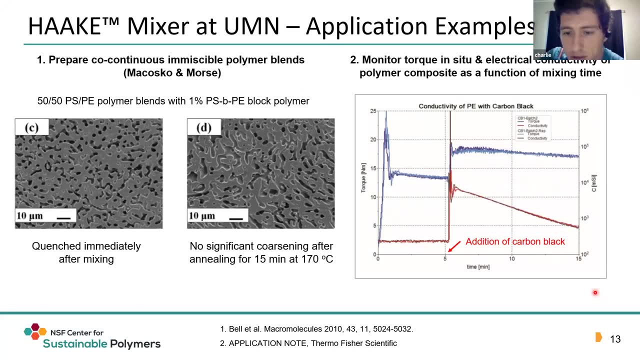 and they used it to prepare polymer blends, co-continuous blends in specific. They added a block copolymer which stabilized the blend, and you could see the results here. Another example of the Hake mixer is: you can use a proper attachment when we don't currently. 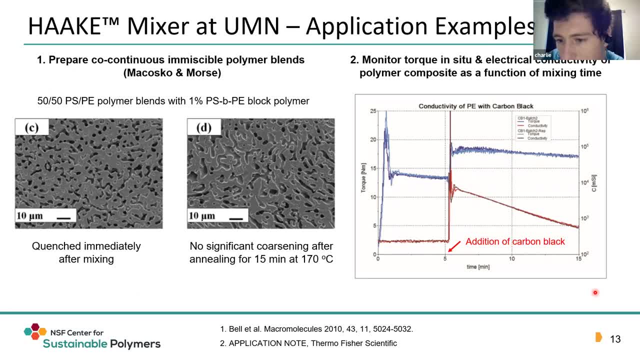 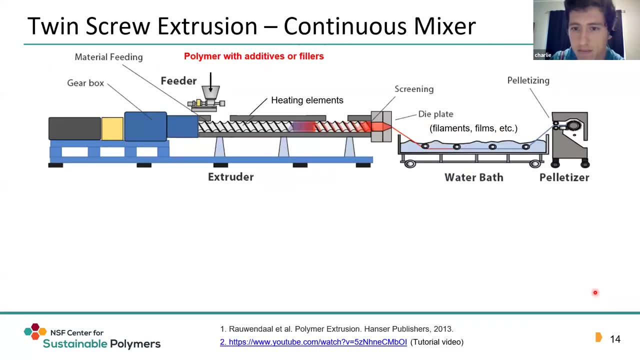 have book head purchase and you can measure other properties in-situ during the melt mixing. Here we measured the electrical conductivity, which is monitored by the addition of carbon black to make a composite is one example there. So next we'll talk about the twin screw extruder, and this is a continuous mixer while the Hake was. 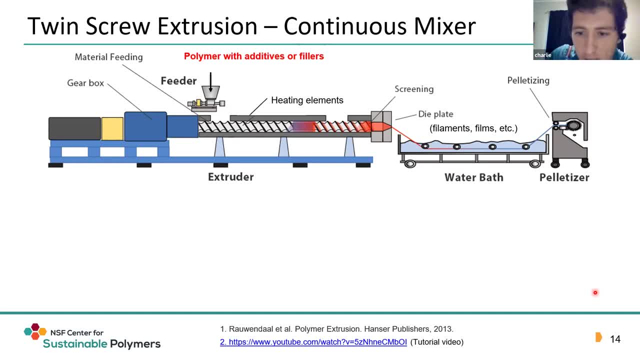 a batch mixer. So we have a mixer here and again you have a feed, so for polymer fillers, additives, and then you have an extruder, a heating block, a die, and then, once the filament comes out of the die, it can then be pelletized if you would like. So now we'll take a more zoomed in. 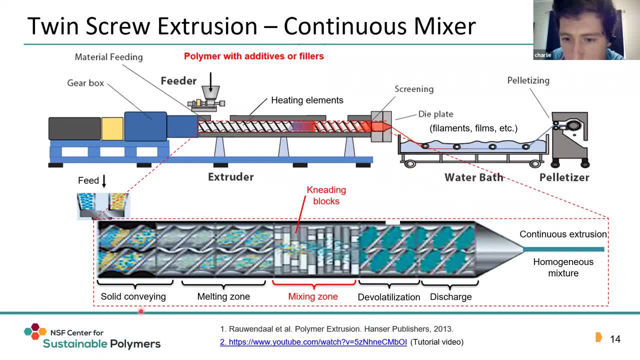 look at what goes on in the mixing section. So in the twin screw you have two screws, you have a conveying zone and a melting zone, and then you have a mixing zone. The mixing zone is where you see those kneading blocks. So you have a mixing zone and you have a conveying zone, and then you 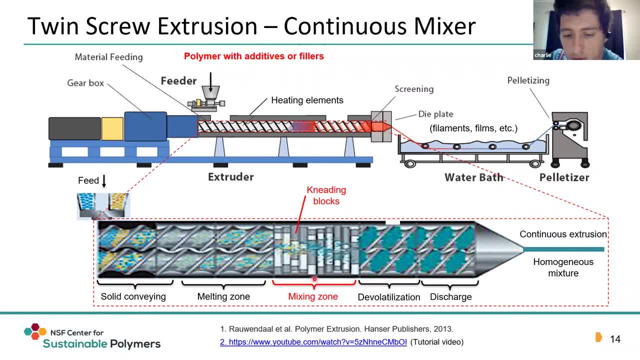 see those kneading blocks which you saw earlier in the beyond the classroom figure, and in these kneading blocks you have. this is where the mixing mostly occurs. So you'll have both shear and extensional flow, and it is very complex. You also then have a degassing zone and then the material. 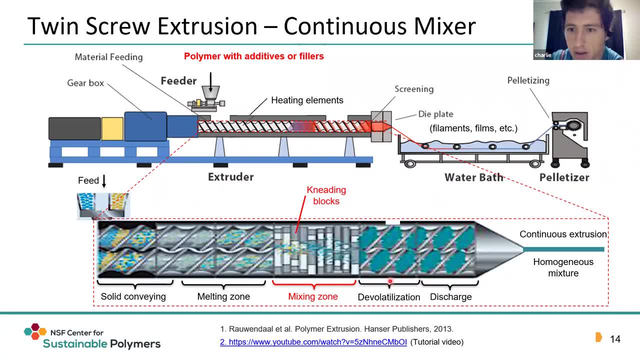 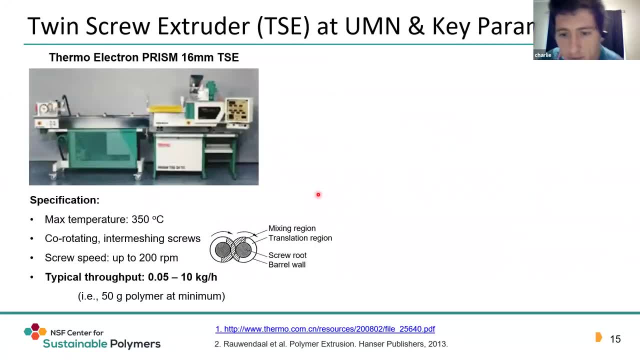 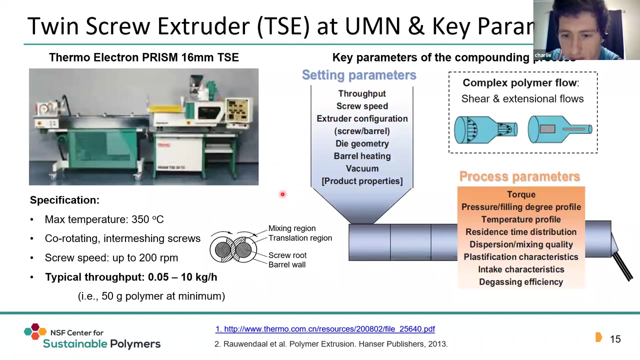 is discharged and extruded into parts. So the specific twin screw extruder we have at the U of M edes is going to have a diluted component. So this is the gigkeiten that we're going to have for the mixing and the combination we're going to have for the mixing, and then the other thing that you'll see is that 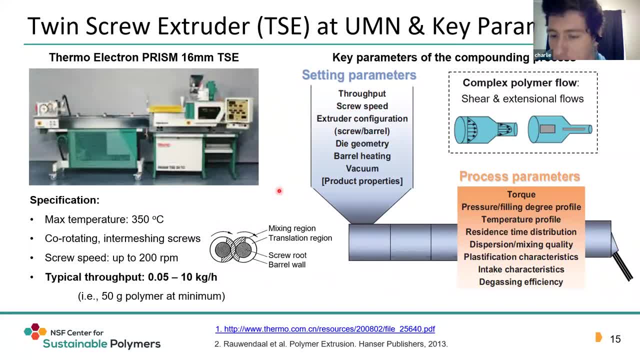 there are also some other renders that have the same convention, and these are the two different, different rinse systems that are used for mixing, and this one is a mix. So, just to characterize it, we're talking about a solid-state mixing system. Here we have a mixture component, which is a. 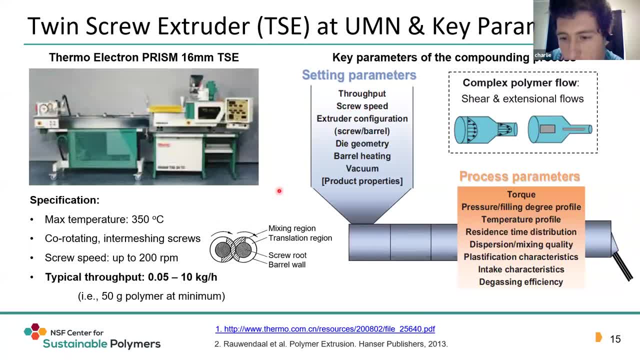 lot of parameters involved with the twin screw extrusion. Some setting parameters are screw speed, screw design and barrel heating. Some process parameters are the pressure profile, the temperature profile and residence time, And I would just like to reiterate that the process 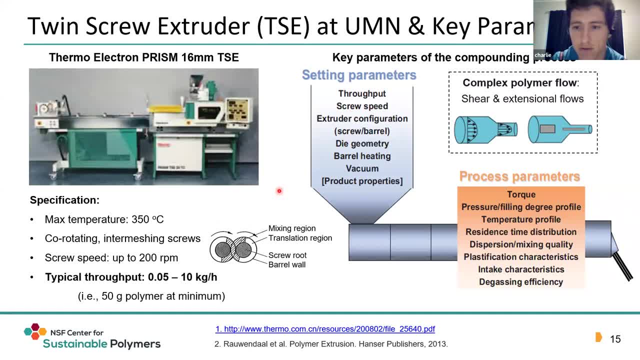 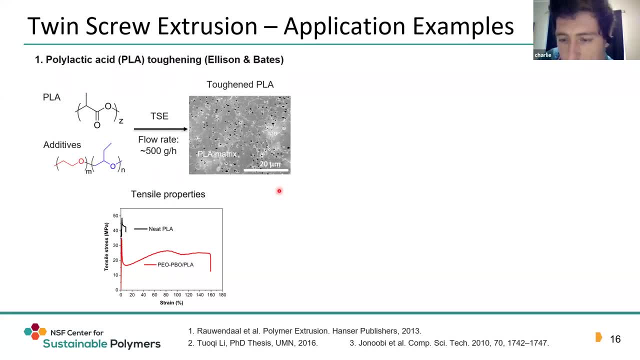 is complex and involves both shear and extensional flows. So in industry a lot of times twin screw extruder is used to make master batches and different compounds. One master batch example from the UMN is from the Ellison and Bates group in which PLA is mixed with a block of polymer. 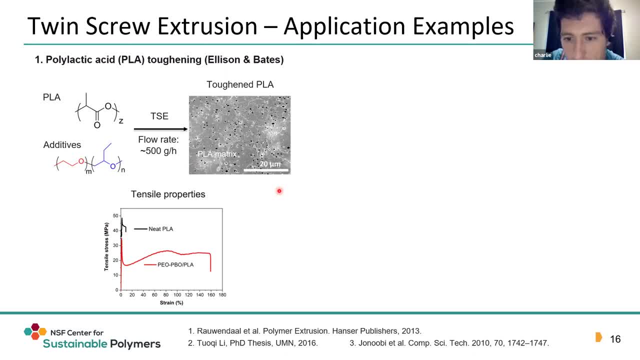 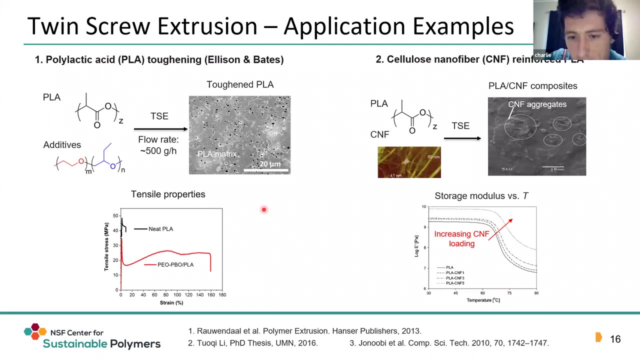 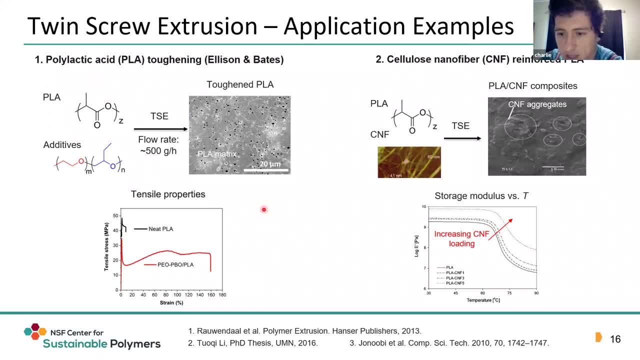 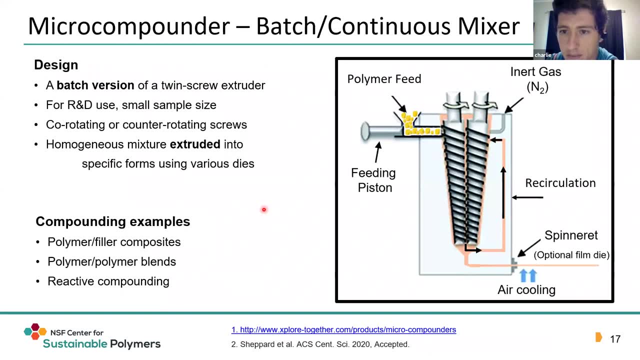 reinforced composite with the cellulose nanofiber And, as you can see, as you increase the cellulose nanofiber loading, the modulus increases. So I've showed you both a batch process and a continuous process, And now I'll show you a process that can do both: the micro compounder. 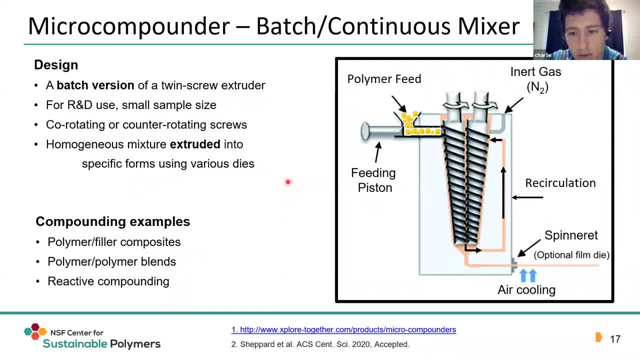 This is a lab-scale version of the twin screw extruder, the previous mixer you just saw, And as it can reach this. So this is the twin screw extruder, which is a twin screw extruder. It's similar shear rates and does similar mixing, but is used for small sample sizes and usually R&D. 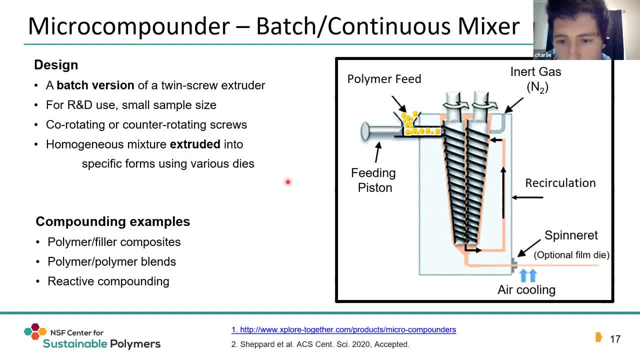 use. So if you look over here on this right figure, we have the polymer feed, conical twin screws for mixing, a recirculation chamber which is to ensure proper mixing, and after your resonance is complete, you can then discharge the polymer out the extruder, and then you can. 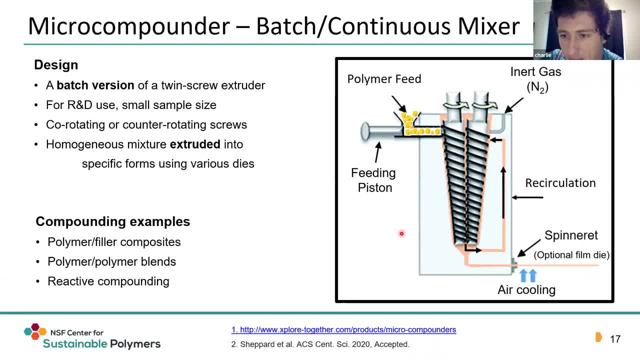 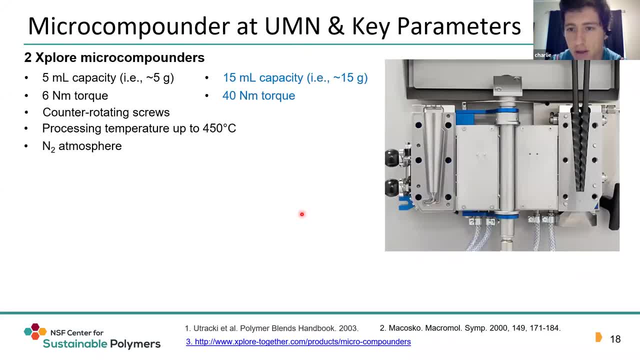 either produce films or a filament, depending on the dye attachment you have. Typically we produce filaments, but I will show you a dye attachment in the future. So at the UMM we have two different micro compounders, one with a 5 milliliter capacity and the other with a 15. 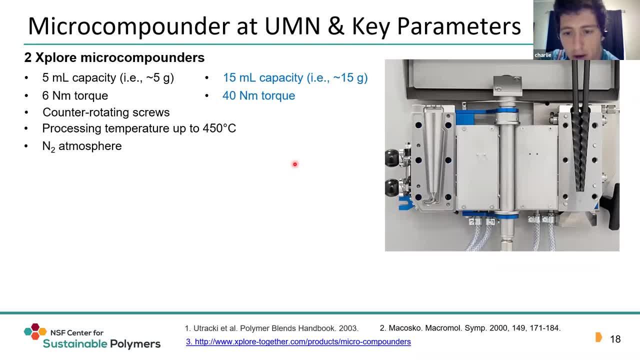 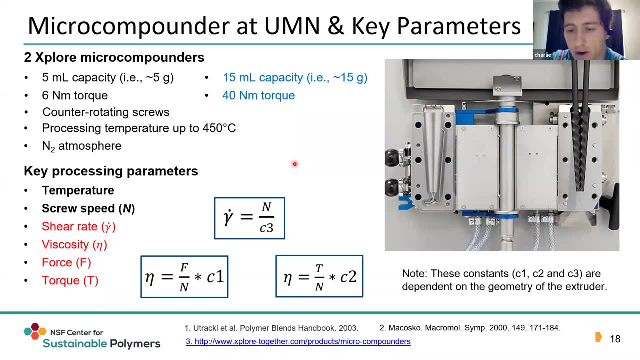 milliliter capacity, and the ones we have at the UMM are counter-rotating screws and they both have the ability to have a nitrogen atmosphere for an inert atmosphere. Some key processing parameters that you can tune is temperature and screw speed. The screw speed can be. 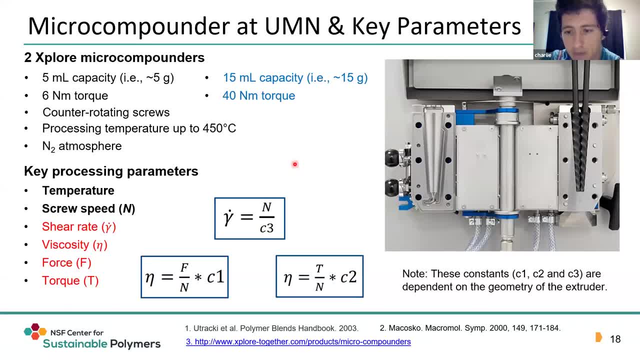 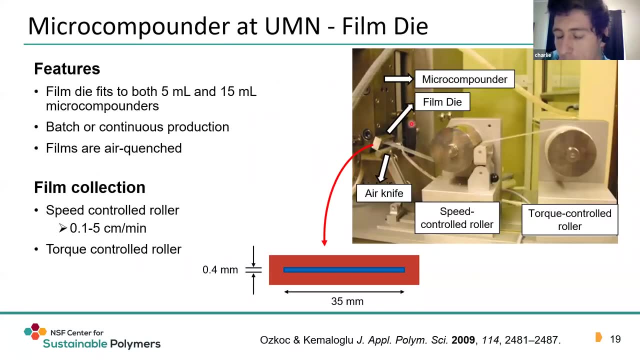 converted to the shear rate through this equation here, and the male viscosity can be measured through the force and torque, as seen there. So again, in-situ measurements can be recorded while mixing. So this is the film dye which you can attach to the micro compounder and you can then extrude. 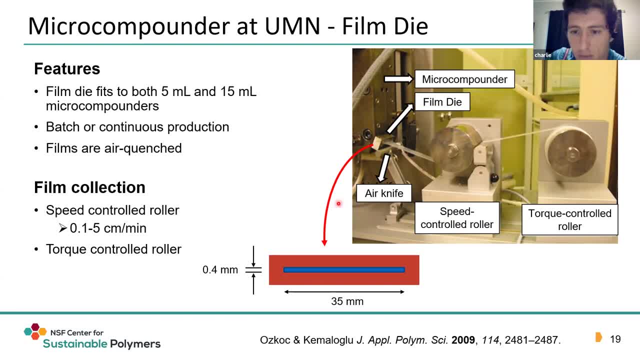 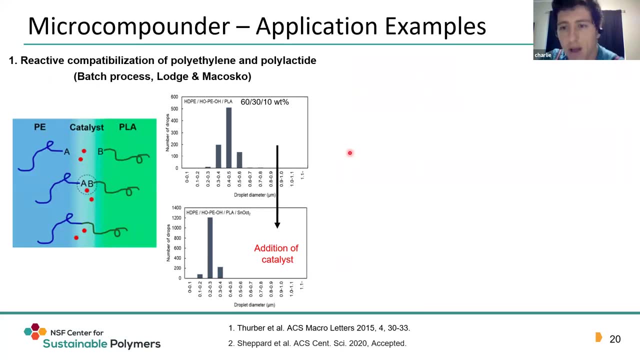 films instead of filament, and the film will come out. Here's my SCARF Match, this little blue section here of the dye, and then the rollers can be used to collect the films. So examples of microcompounding from the UMM are so, the first one here. 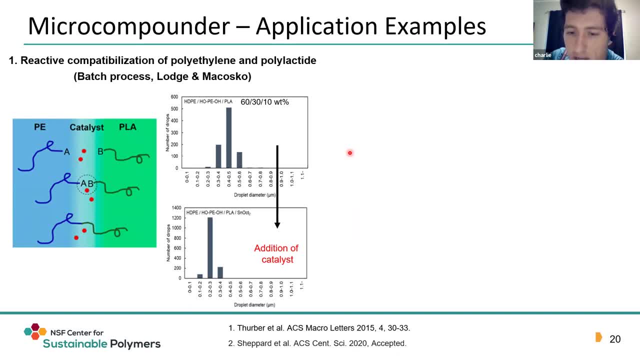 is from the Lodge and McCaskill Group, in which a batch process was used. So there they used a reactive compatibilization of poly-ethylene and PLA blends, in which they used ordinary. they added a catalyst, and because the catalyst was added, 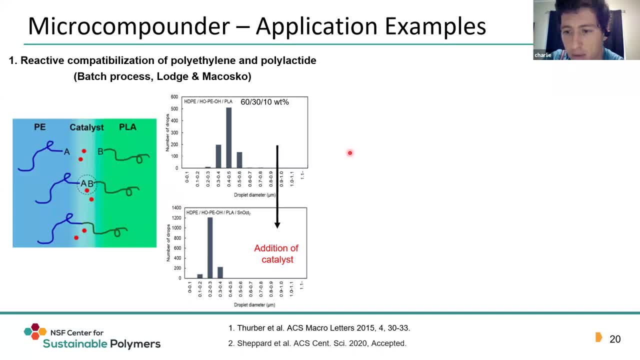 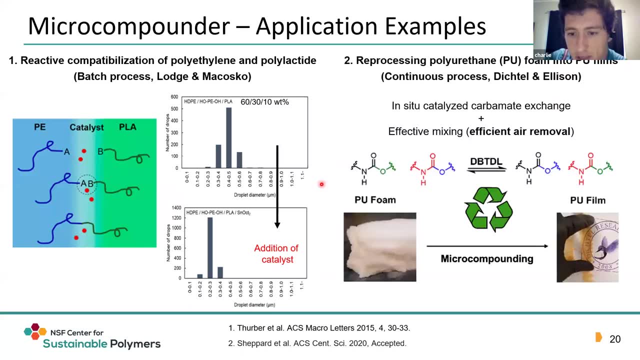 a reaction happened at the interface of the two polymers and formed blocko-polymers to reduce the interfacial tension And therefore you could see the dispersion size decreased. A more recent example, one from the CSP, is a continuous process of polyurethane foams. 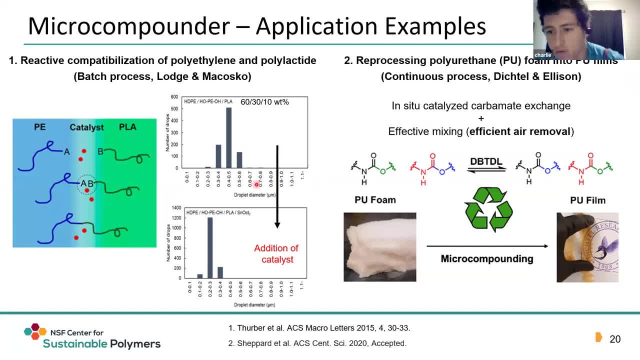 So the microcompounder proved to be an effective way to remove, as well as an effective way for the to enhance the carbonate reaction in situ, And it turned cross-linked polyurethane foam waste, and then we're able to reprocess them into films. 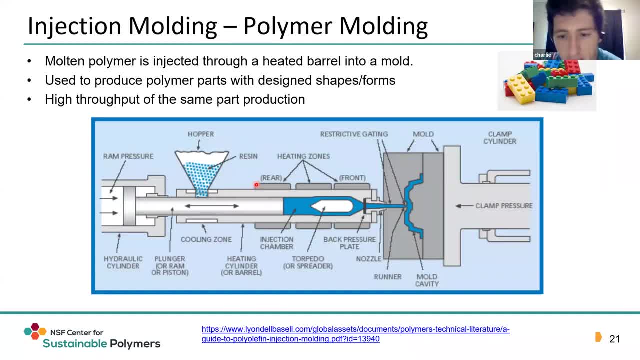 So this is now the molding part before we talked about the mixing. So the previous process equipment was associated with mixing and injection And this is going to be the injection molder which will take those mixed polymers and make the final products with them. 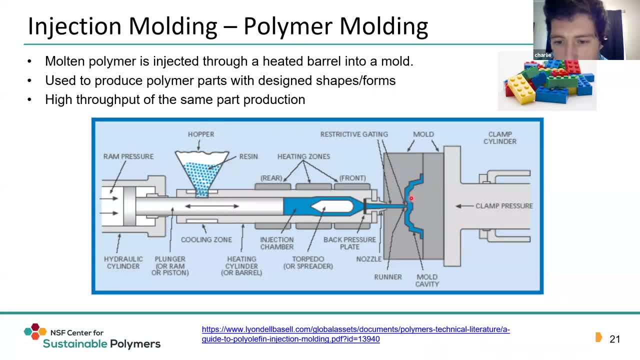 So for this machine, polymer is fed into the hopper and then there is a heated barrel with which the material is pushed through with a piston and it will be filled into a mold. So this process is used for high throughput of the same part. 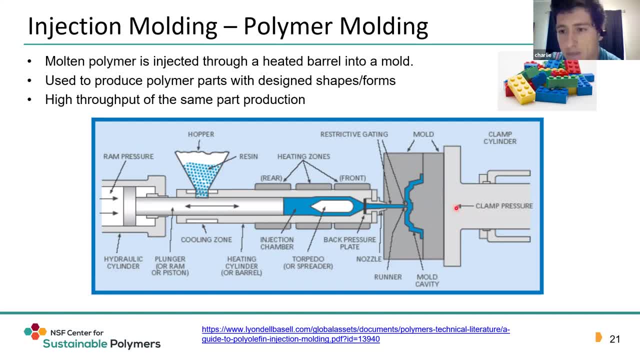 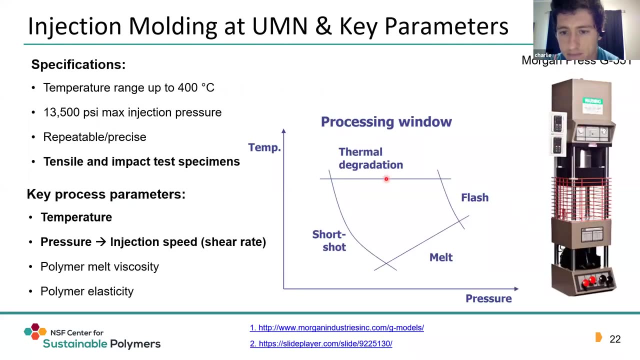 and you get very tight tolerances. So one material that's made this way are Legos. One disadvantage is that you need to machine and mold. you need to machine a mold, which could take time and is also expensive to make. So key parameters for the injection molder. 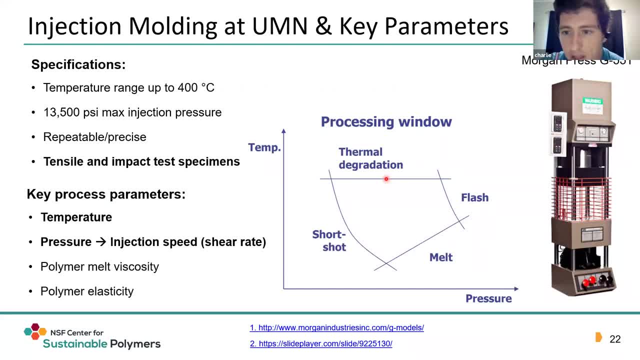 are the temperature and pressure. So if you don't have the right temperature and pressure, you're going to either overfill your mold or underfill your mold and you won't have the proper product. At U of M two particular molds we have. 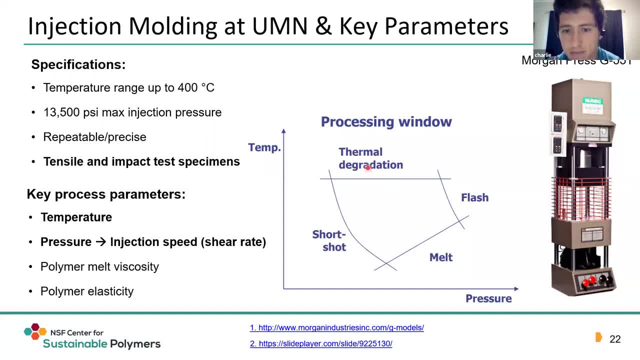 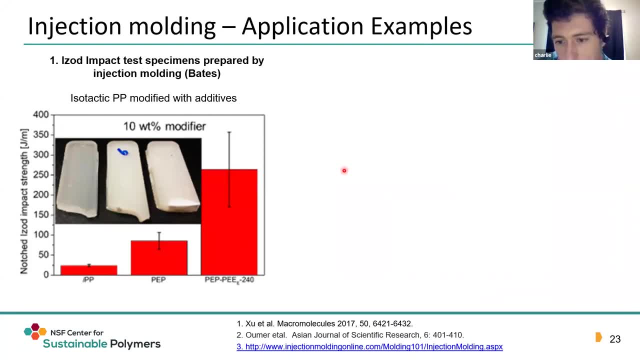 are a tensile bar and an impact test specimen. So one example of using the impact test specimen was in the Bates group, The injection molded to produce IZOD impact test bars, which was IPP toughened with Block O Palmer, and then they were able to test all these impact bars. 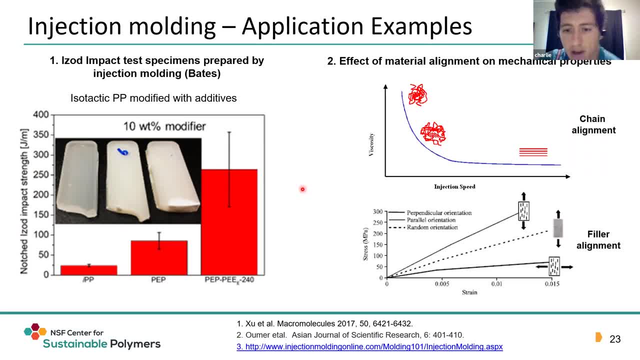 at a very efficient manner. And another way. another thing the injection molding is used for is to study the effect of the chain alignment of fillers- and just physical, you way, Okay, the chains- and see how it impacts the material properties. all right, great. 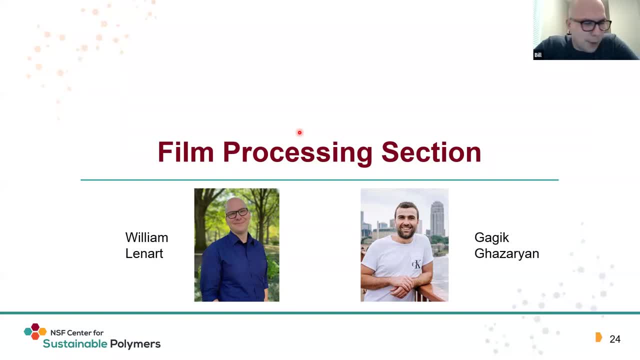 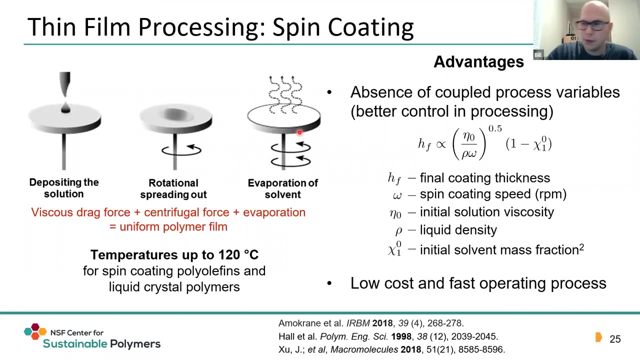 thank you. my name is William Leonard. I go by Bill. I am a recent postdoc with the Ellison group. I started with them just before everything started shutting down, so it's great to be here with you all to be able to talk about some film processing. so often, when you create a material, you want to characterize it in. 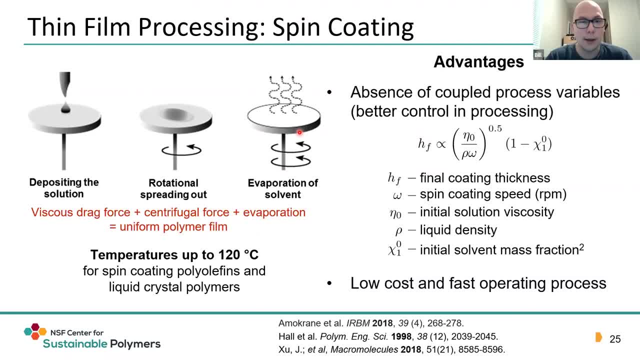 solid state. it's very frequent. you want to make it out of a film, and one of the easiest ways to do that is to dissolve it in some compatible solvent and then spin coat it, where you use a high-speed rotating substrate, and then the solvent evaporates, leaving behind your polymer film. and what's helpful about this is 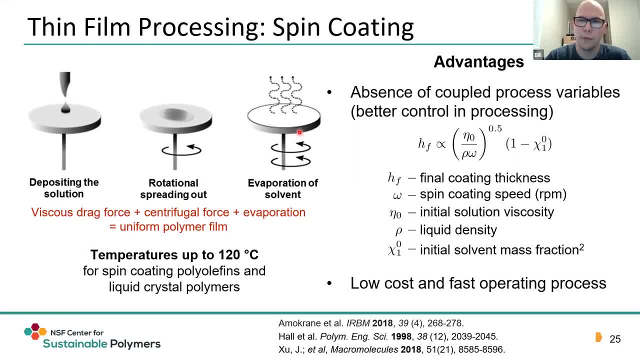 that's pretty easy to tune the height of your film from some of these independent variables based on your solutions, viscosity and how fast you're rotating, and one of the unique capabilities we have here is to do high temperature spin coating, which allows for the us to make polyolefin films or liquid crystal. 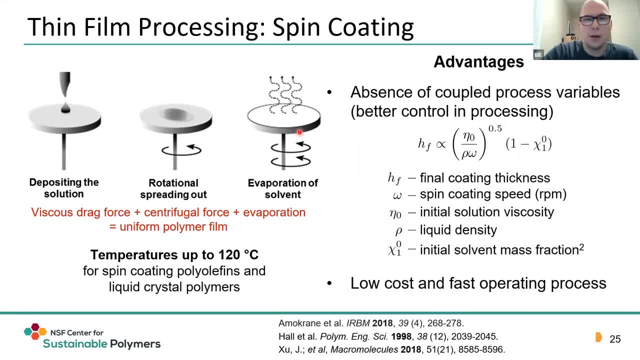 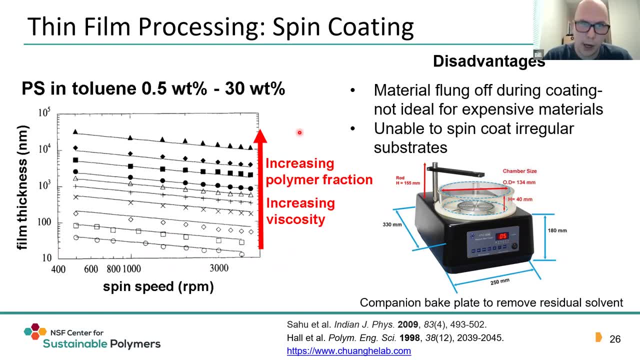 polymer thin films as well, next up. so really, when you the things you need to think about when you're making these types of films is what polymer fraction you're going to use and that increases the viscosity of your solution and that gives you a kind of a base limit on what thicknesses you're able to actually. 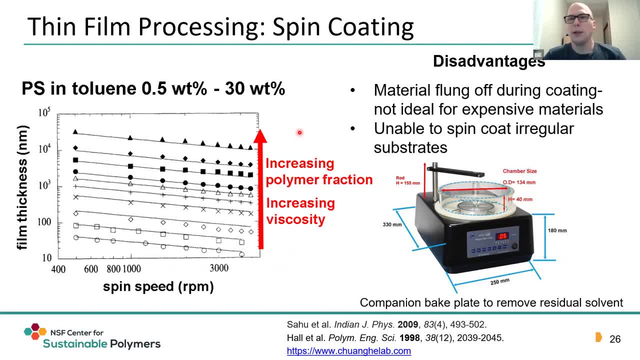 access within the RPMs of the system. and some of the limitations here beyond that is you do lose material. so if it's very expensive it might not be the most ideal. you might just want a regular, just casting then, and then really it's not able to spin to coat irregular substrates and in addition we do have a 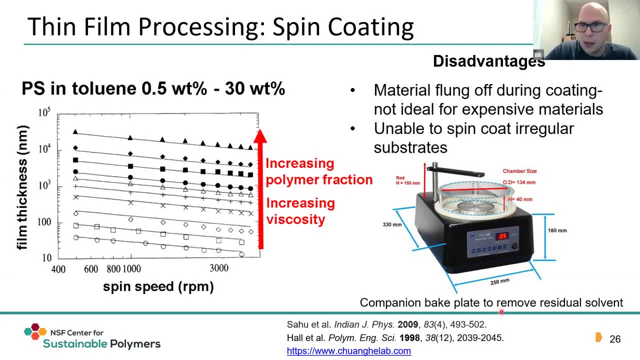 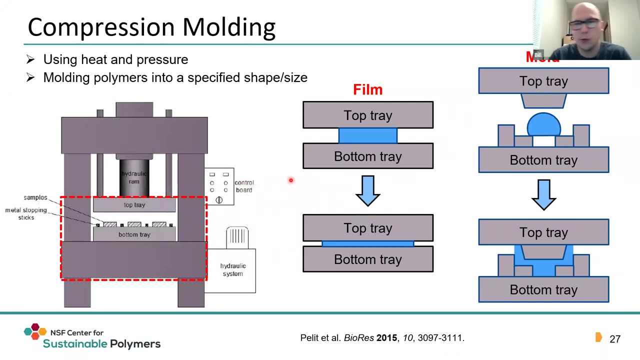 companion bake plate so we you can remove any residual solvent to finish drying your sample for further characterization. next slide. next slide, please. so one way to mold a polymer film to an irregular substrate is with compression molding, and this allows you to access either regular kind of thicker films from the melt exclusively. there is no need for. 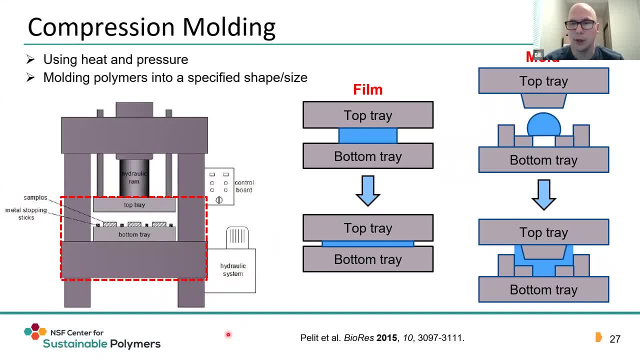 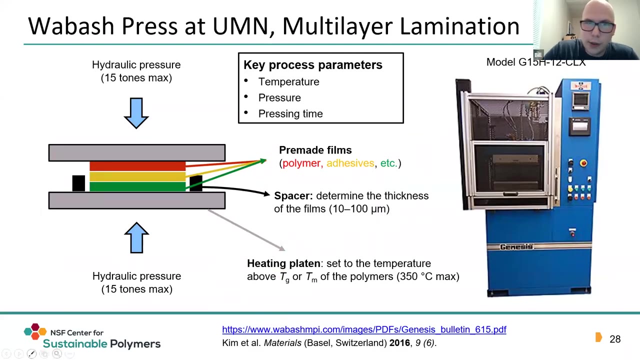 a solution or a solvent, and then it does allow you to get some basic irregular shapes as well, and the main parameters you have here controlling your sample properties are your heat and pressure, and then your hold time and some of your cooling characteristics. next slide and then what you further. where you can do with this is if you have some pre-made films either. 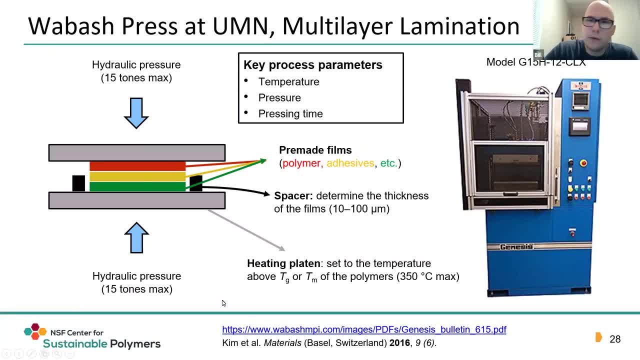 made from spin coating or from pressing them as films. previously, with the compression molder you can laminate films and look at adhesive properties, diffusion between the layers or some other interactions at the interface that you might find interesting. and again the same kind of controlling parameters. is your temperature, pressure, pressing time and you want to consider the TG or TM of the materials. 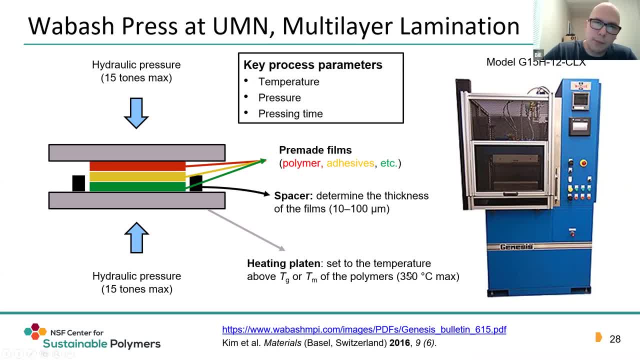 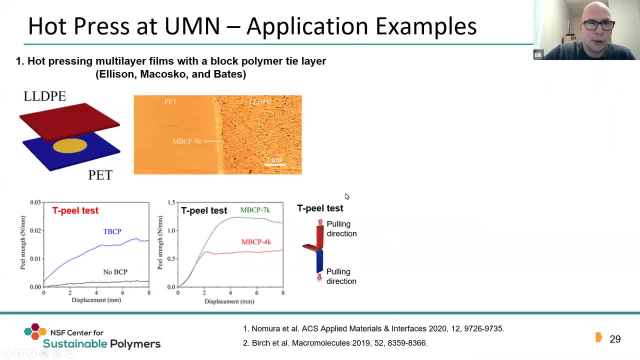 that you're working with to kind of derive what process parameters you want to use. and so a specific example of what's been done here is the use of a black hole polymer to act as a tie layer for uh between two pumping incompatible polymers, where we see a substantial increase in. 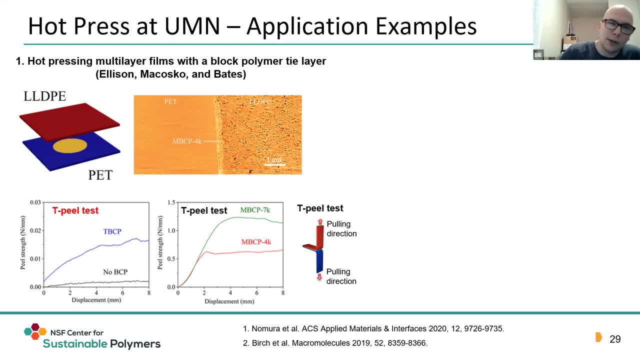 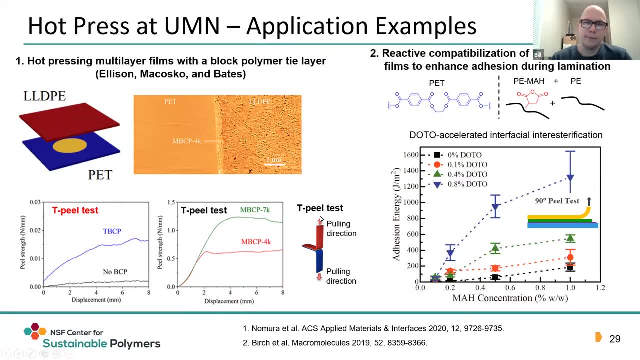 adhesion, uh, between the two phases. with this inclusion of the blo FT polymer that kind of entangles with both phases and ties them together. and then additionally looking at React, of compatibilityization. so The diffusion of the two phases causes the reactive groups on each polymer to interact and then you get adhesion as well, without the need to include a third phase such as the block of polymers previously. 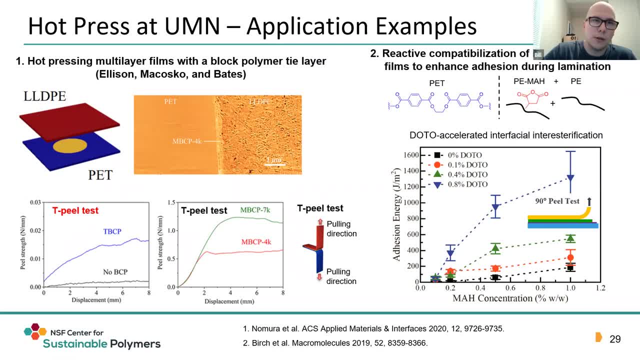 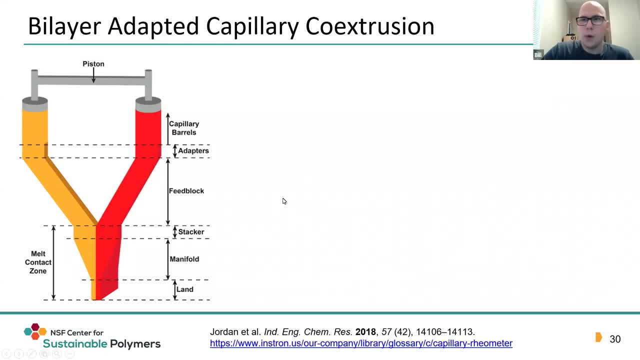 So it's a kind of an in-situ method to compatibilize two incompatible materials. And another kind of way to make thin films, specifically a bilayer system, is the use of our capillary rheometer with two barrels. that allows you to co-extrude two films together, two polymer melts together, 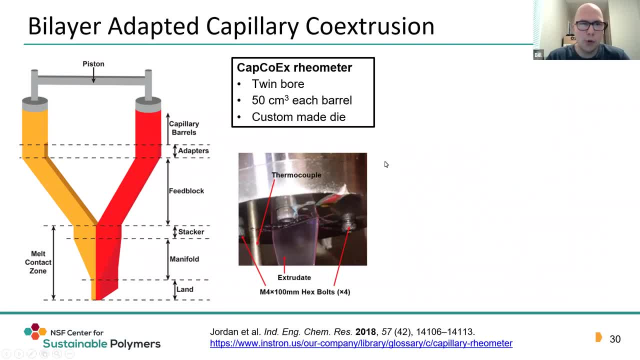 where each. the kind of limitations here is that each bore must be at the same temperature and piston speed. So you do have some limitations there that will alter kind of your melt contact time A little bit, And then we're able to access a fairly wide range of interface contact times to examine kind of in-situ reactions or, if you're interested in localization at the interface, this might be a good small-scale method for you as well. 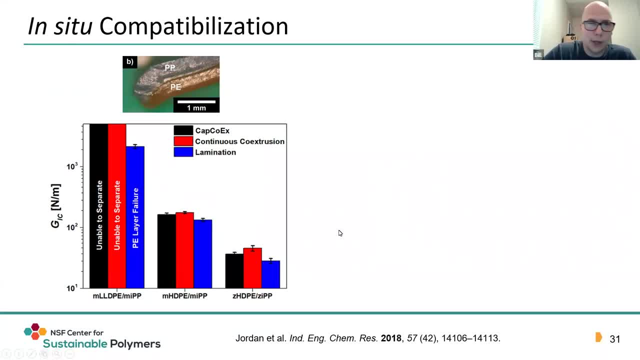 So some things that's been done here is kind of in-situ compatibilization, where we've examined kind of the effects of the polymerization type Of the polyolefin and how they inter-diffuse with each other, showing and then also reactive compatibilization, showing we get better improved adhesion with this increased contact time, allowing you to kind of better understand scaled up process parameters. 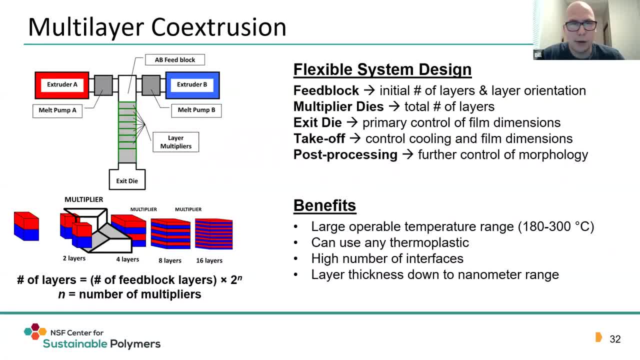 And another kind of step up from that. if you're looking for a higher number of layers or a higher number of interfaces, is multi-layer co-extrusion. This is a much larger scene. So if you're looking for a higher number of layers or a higher number of interfaces, is multi-layer co-extrusion. This is a much larger scene. So if you're looking for a higher number of layers or a higher number of interfaces, is multi-layer co-extrusion. So if you're looking for a higher number of layers or a higher number of interfaces, is multi-layer co-extrusion. 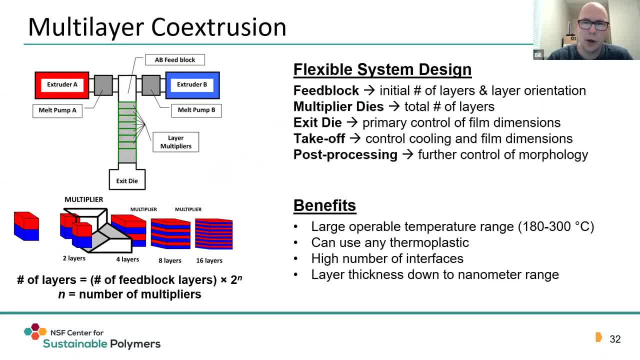 Each extruder you need about 500 grams for, And then it does have a fair amount of flexibility beyond that, where you can control your number of layers, either from the onset at the feed block, with the addition of layer multipliers, And then you can control your film size and thickness with your takeoff, your exit die and any other post-processing that you might be interested in. 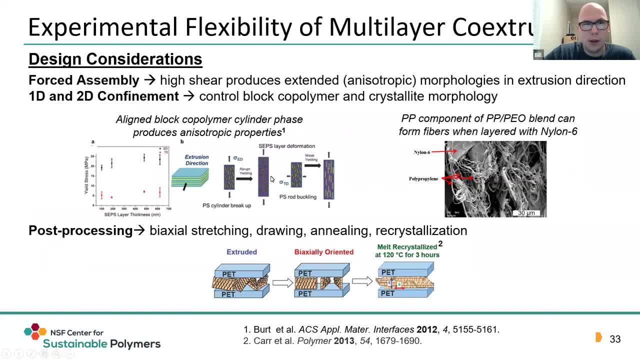 And so some of the special design considerations. here is the combination of the high shear and layer confinement that allows you to kind of get this forced assembly. So for example in a block copolymer system, alignment of a cylinder phase with the extrusion. 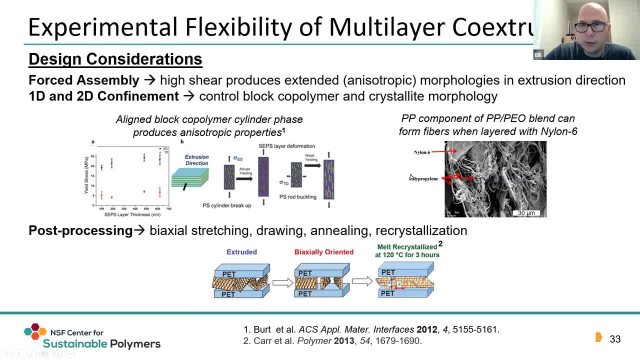 direction and in a blended phase of polypropylene and polyethylene oxide, you can actually get the polypropylene to form a continuous fiber forming phase And then further processing can be done on these systems to control the morphology with the confinement effects beyond that, giving you a 2D confinement instead of the 1D confinement. 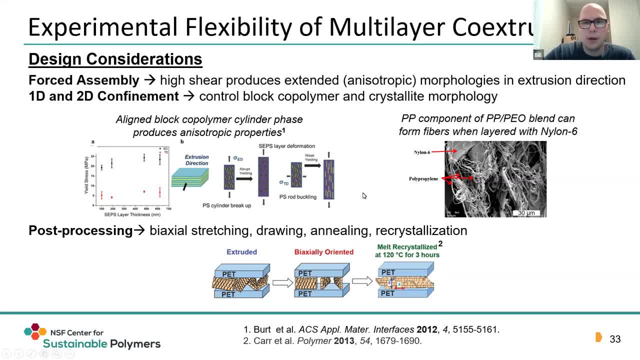 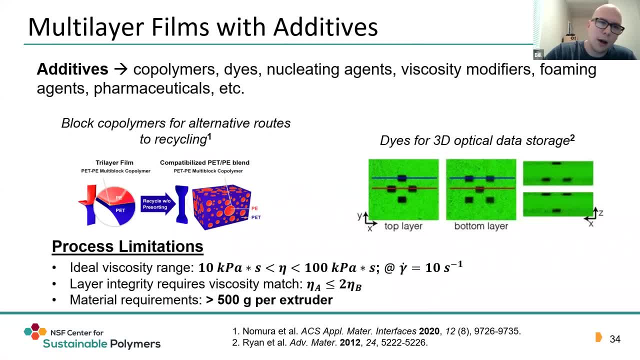 you typically see from spin coating. And additionally, you can add a variety of additives to the system where, going back to that previous work, You could add block copolymers. There's an alternative route for recycling: You could include dyes. 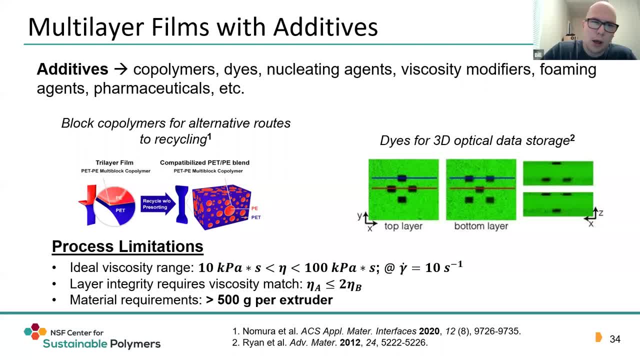 Dyes have been included for 3D optical data storage. Really, the only restrictions you have in the process are: you want kind of your system to be in this viscosity range between 10 and 100 kilopascal seconds at this shear rate, And that gives you good layer integrity. if your viscosity then is within two times of 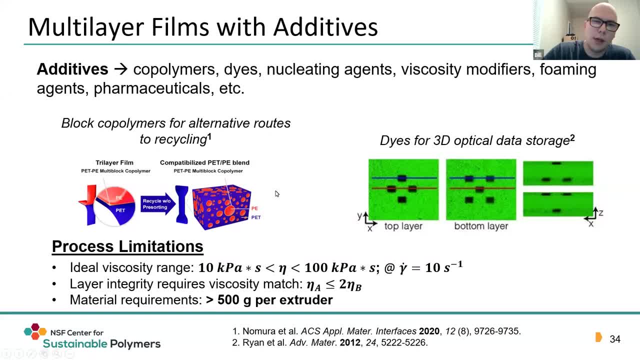 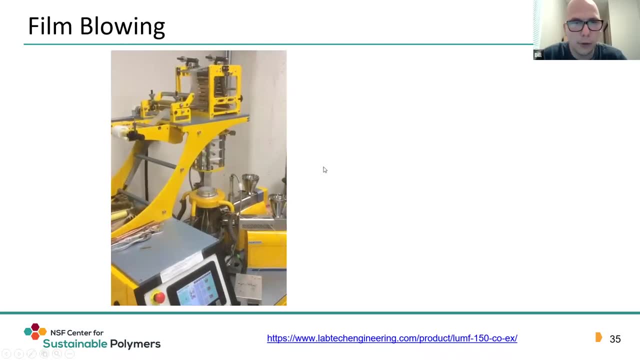 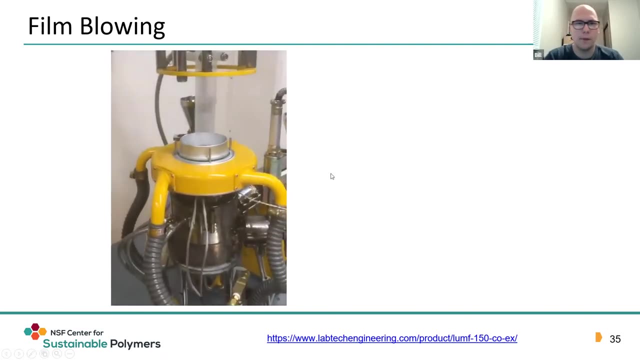 each other. So you're getting consistent layer thickness, Yeah, And throughout your whole system. But then again you do have high sample requirement here And kind of this. last more unique system we have is this small scale film blowing system. This works on a similar capacity as the multilayer co-extrusion, about 500 grams per extruder. 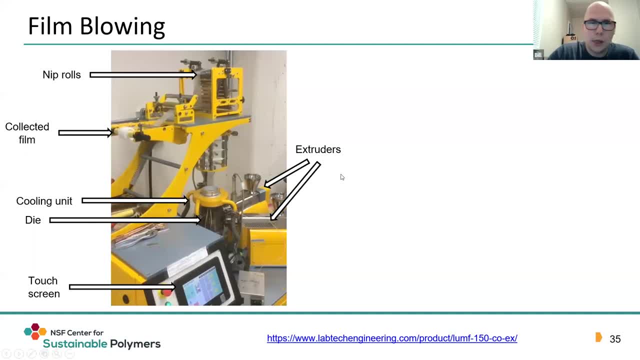 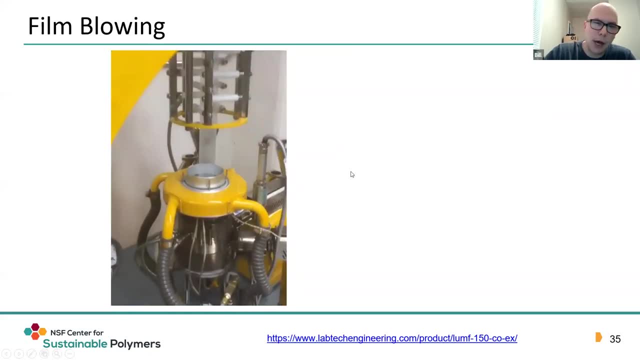 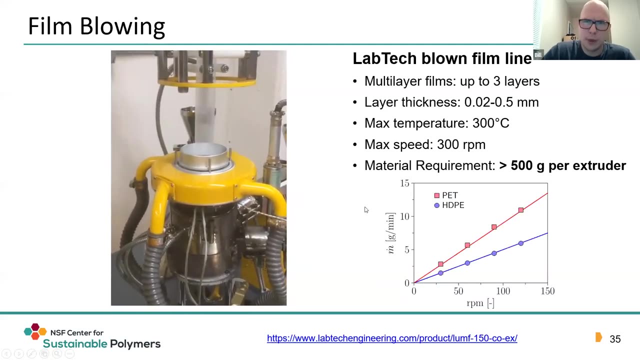 And we're able to actually have three extruders here, So we can layer three polymers together, Either one as a tie layer to looking at compatibilizing or adhering to incompatible polymer systems. together You can look at effects that blow up on your system. 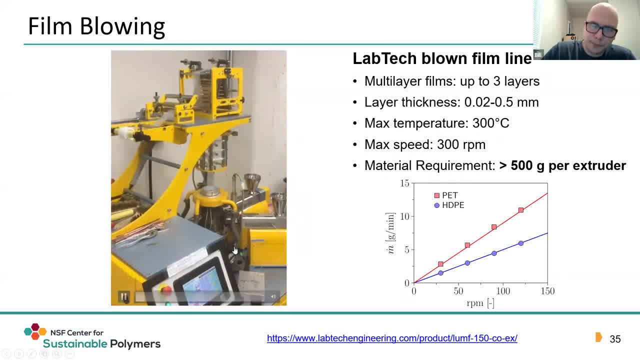 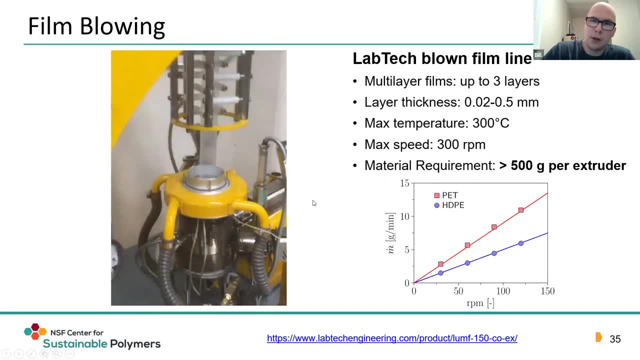 And we have pretty good control over the relationship between the flow rate and the operating speeds of the equipment. Thank you, Hi. Good afternoon everyone. My name is Anirudh. I'm a professor at the University of Michigan. I'm a professor at the University of Michigan. 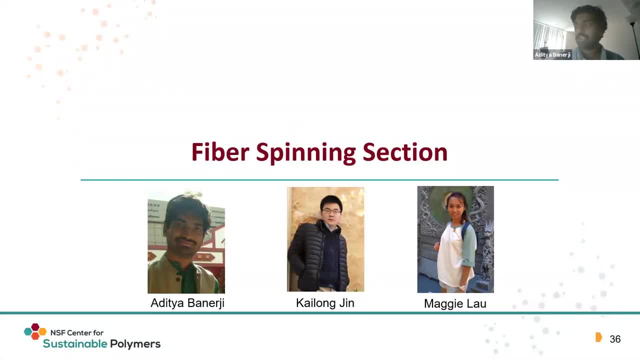 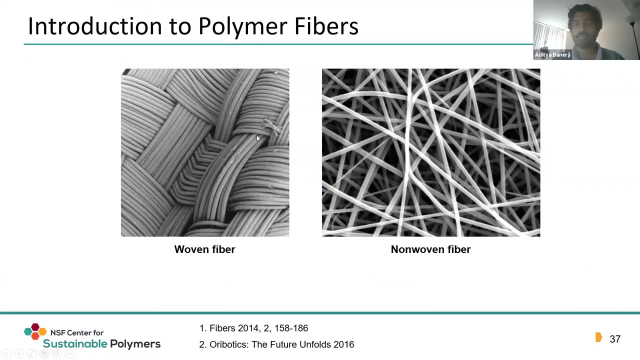 I'm a professor at the University of Michigan, My name is Aditya, I'm a graduate student in the Ellison group And in this section I will be talking about how the processing techniques are used to make fibers. So if I move to the next slide, just as a broad background, the typical types of fiber. 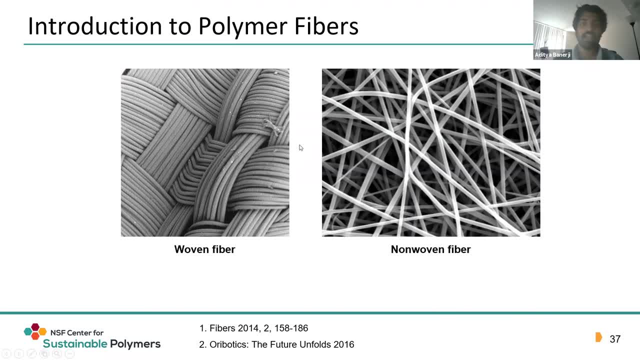 mats that are produced from polymeric feedstocks are broadly categorized into woven fibers and nonwoven fibers, As the image is showing here, the polymers that are produced from polymeric feedstocks. they are performed by the independent ο-contracts, which is a polymers that we use in the coding process, or polymers that 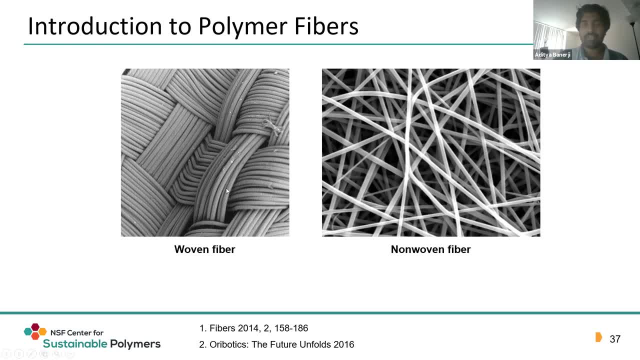 are used by the independent groups, And this does not mean that they are not voluntarily molded as Sol-O-Magic or Polymer fiber, But it does suggest woven fibers are those in which the individual fibers are stitched in a given pattern, while in nonwovens the fibers are laid down randomly on top of. 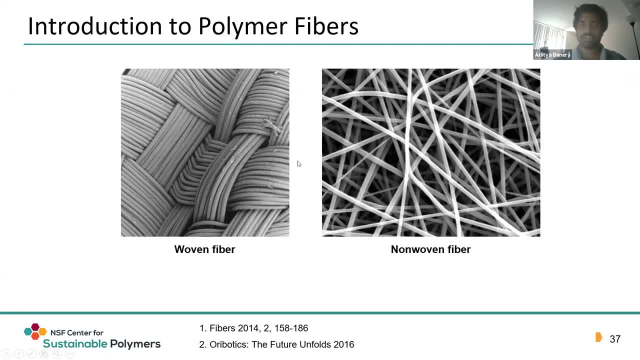 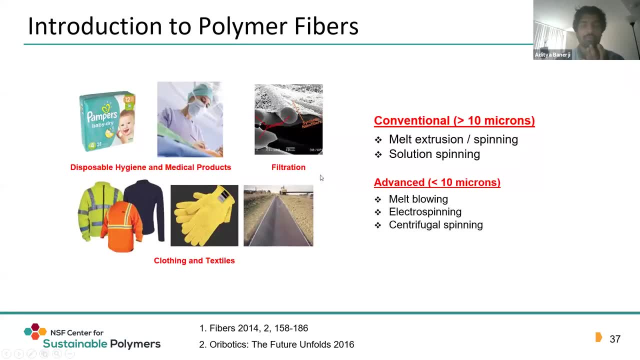 each other, which are held together by physical interactions, or in some cases they are also chemically bonded, for mechanical stability as well. So some of the applications which are very commonly used for fibers, as well as different types of fibers for fibers, include disposable hygiene and medical products, For example, in this current COVID. 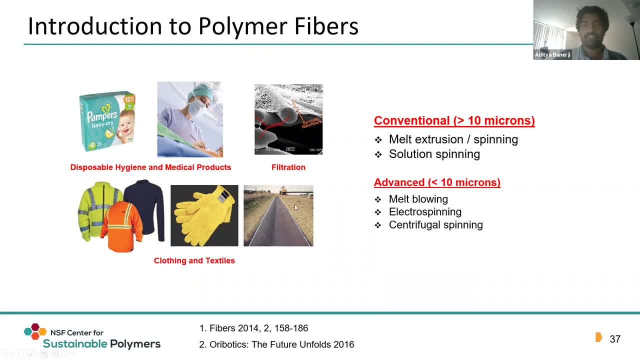 outbreak, you would have seen so much a demand of N95 masks. The main material of the N95 mask is basically a non-woven mesh of polypropylene. In addition to those disposable hygiene products, there's a vast demand of these polymer fibers in filtrations, as you can imagine as well. 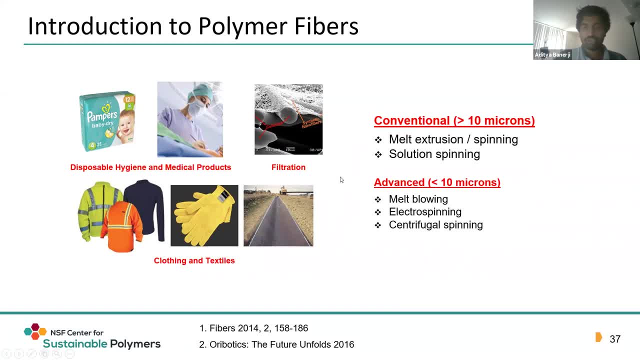 in clothings and textiles, as these people suggest. So some of the techniques in which these polymer fibers are generally made include conventional methods like melt spinning or solution spinning, in which typical fiber diameters are above 10 microns or so, while 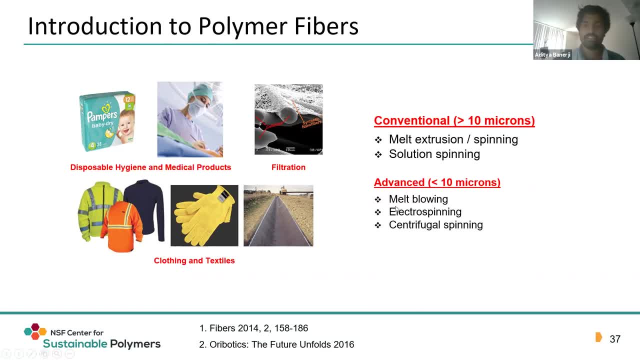 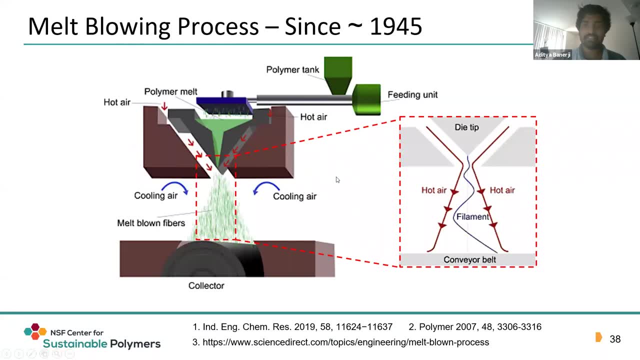 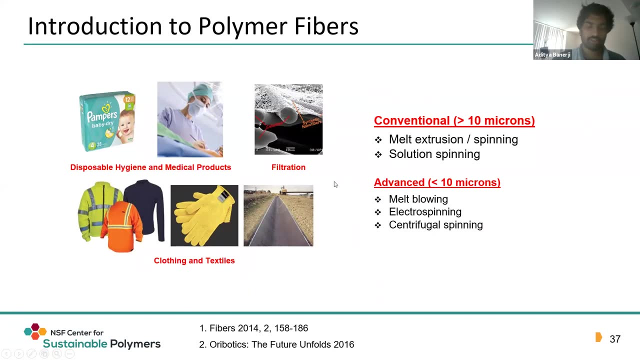 the advanced methods involve melt, bluing and electrospinning, in which fiber diameters much less than 10 microns, even in the range of nanometers, are attainable. The major difference between the conventional and the advanced process is the way the fibers are. 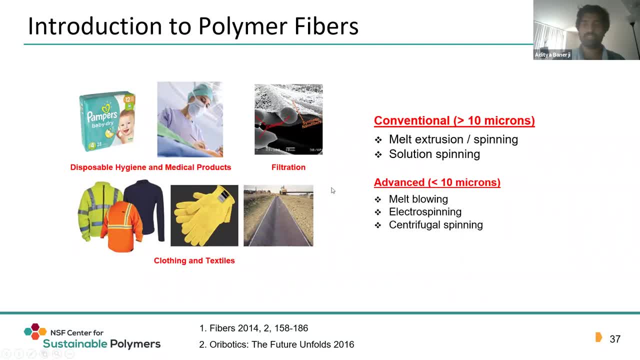 drawn out and also the viscoelastic property of the polymers that are used in these particular processes. For example, in conventional methods the fiber is drawn by a mechanical takeoff wheel and winding. that happens afterwards, which leads to the much higher diameter that is. 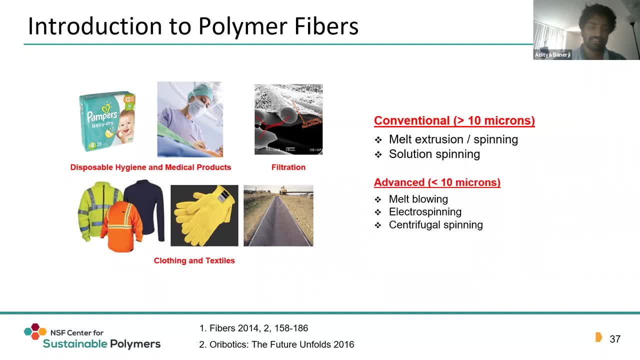 obtained In comparison. in the advanced methods there is additional drawing force, For example, high-velocity air jets in melt blowing and electric field in electrospinning, which leads to much higher stretching of the fiber filaments, leading to much smaller diameter. In addition to that, from a viscoelastic point of view as well, the advanced 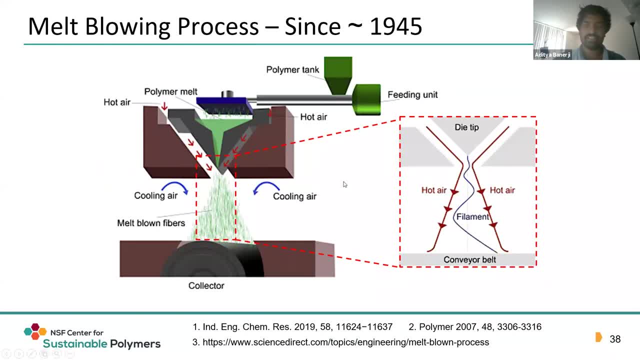 methods typically involve much lower viscosity and elastic properties, leading to those particular diameter ranges. So the two processes that I would be focusing on are melt blowing and electrospinning. As you can see, melt blowing has been commonly used in the industry for about half. 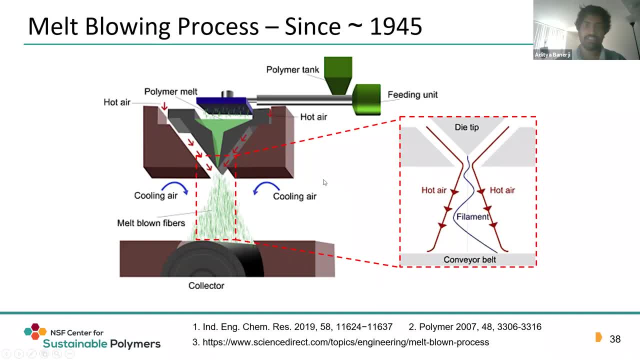 a century. right now, How it operates is basically: the polymer is fed through the green hopper at the top and once it passes through the dye, it is melted at high temperature above its glass transition temperature or its melting temperature, which is extruded through the 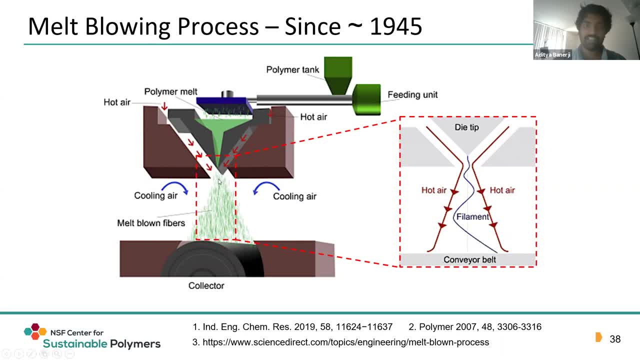 dye tip and the red. the hot air jets marked by the red arrows stretch them out into thin filaments, leading to further thinning and reduction in diameters, which, during flight, cools down and cools down below its solidification temperature and is subsequently collected down. 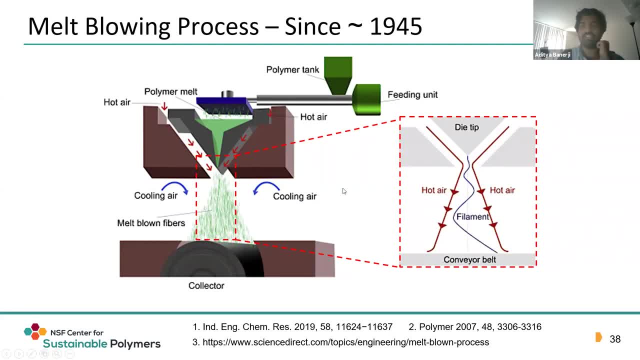 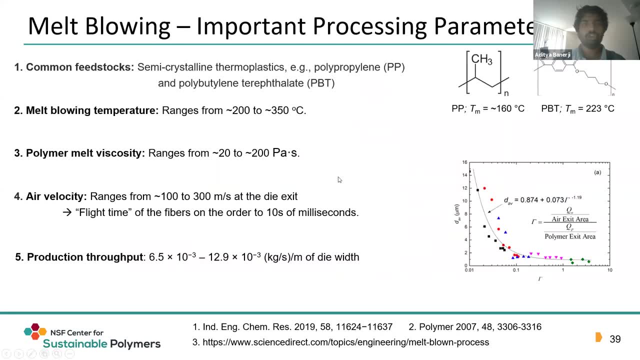 below in the rotating drum, The inset on the right basically highlights the mechanism by which this particular process is happening. Some of the common feedstocks, like I mentioned in case of N95 mask, is like polypropylene and polybutylene terephthalates, which provides a high melting temperature, which basically gives 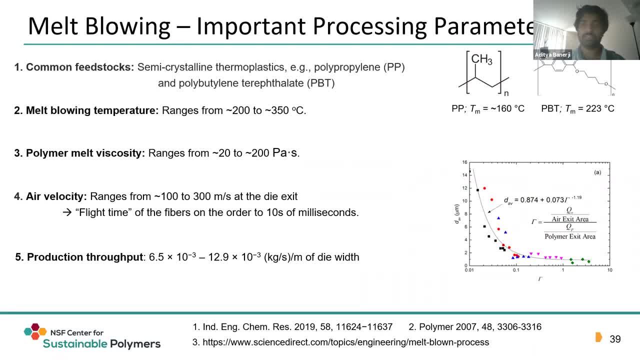 at the upper ceiling temperature up to which that particular polymer fiber are stable. The typical mild blowing temperatures are in the range of about 200 to 350 Celsius, while the viscosity ranges about 20 to 200 Pascal seconds. for optimum performance as well. 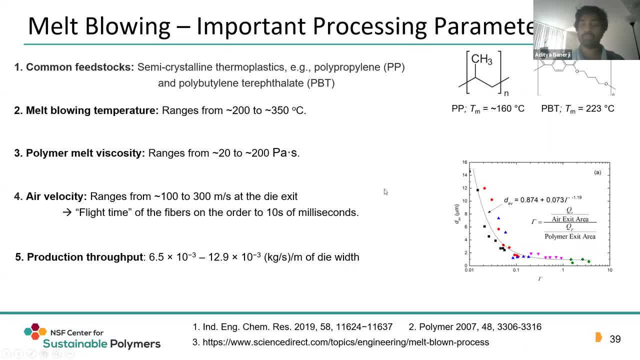 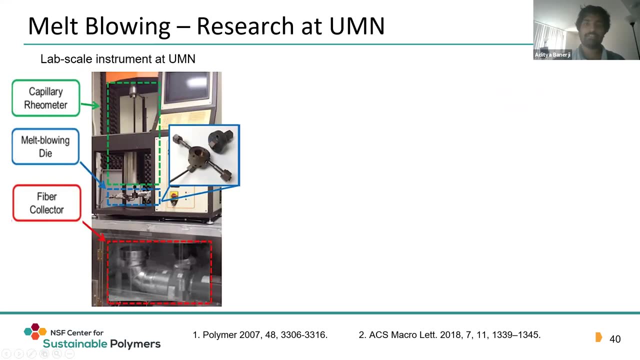 And, as you can see from the feed bullet point, the product. it's a high throughput method as well, which leads to a larger, large scale production of polymer fibers in the industry as well. So, moving on to the next slide, this is the particular equipment that we have at UMN in. 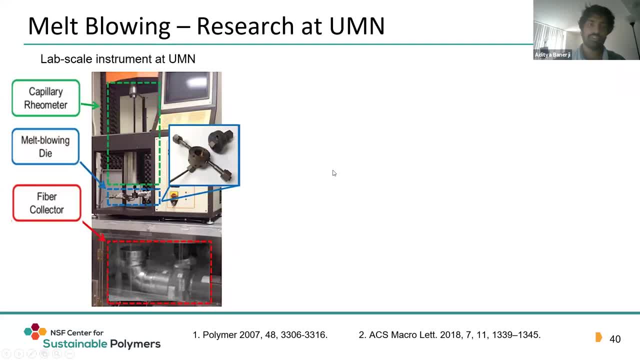 Amundsen Hall, in which a capillary rheometer is attached to a mild blowing dye, which is shown in the blue inset. The capillary rheometer serves the purpose of pushing the polymer melt through the mild blowing dye, which then, as I mentioned, gets drawn down into fibers. 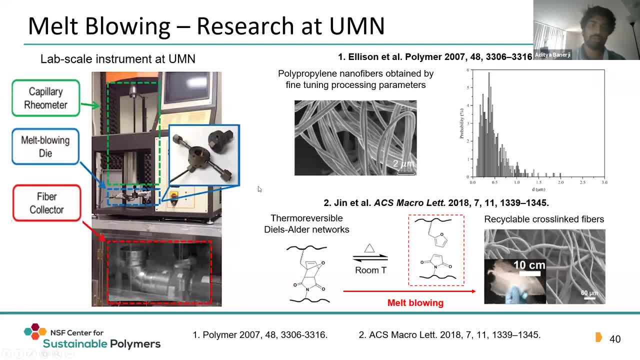 thin fibers, which are collected in the bottom section as well. So a couple of research areas that has been studied in UMN includes the first one, in which polypropylene was used to produce nanofibers by fine tuning certain processing parameters. 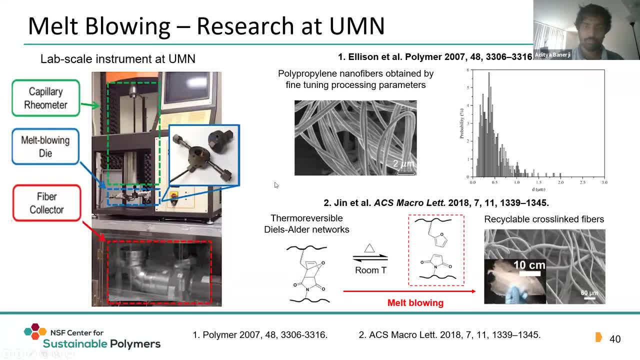 like the viscoelastic properties. In terms of polypropylene-produced materials, there are several 1800 milliliters produced and in the following year has only been found onto alla fiber, And the polypropylene에요-produced materials were excluded in the stock. 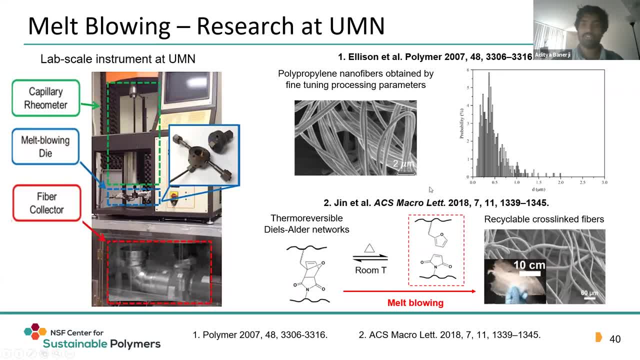 and for aichi version. the polypropylene has been inconclusive and has to be stripped or tanned into a mireけどleiments of this form. The volumeеюсь-produced moment, is veryvoltage when free of сп strongly, which is a. huge disadvantage. Already, after 10 years using ethyl polypropylene, we about 5,000 units of DNA- ordinary and �ple'd the most recent- weren't considered as a nicole cortical surface. So at least 15 years previously we didn't see any. during the first phase of the 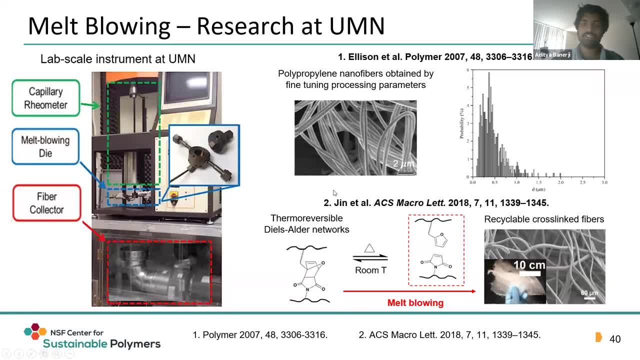 players. We are a growing, bigger population as the mass 7000 Uh K forts, But while we are also thermo-reversible, deals on the network can provide a method in which you can get recyclable cross-link fibers, which also leads to a sustainable aspect of this particular technique. 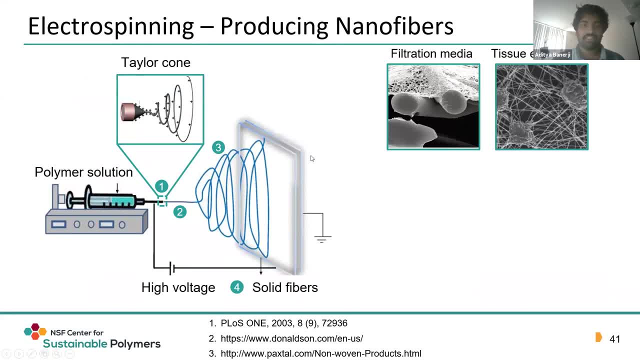 In comparison, in electrospinning, in contrast to polymer melt, in electrospinning polymer solutions are used which are drawn into thin fiber jets using strong electric field in the range of about 10 to 50 kilovolt or so, And due to the high stretching force that is available for this, the typical fiber diameters are in the range of one microns or even lower, in the nanometer scale as well. 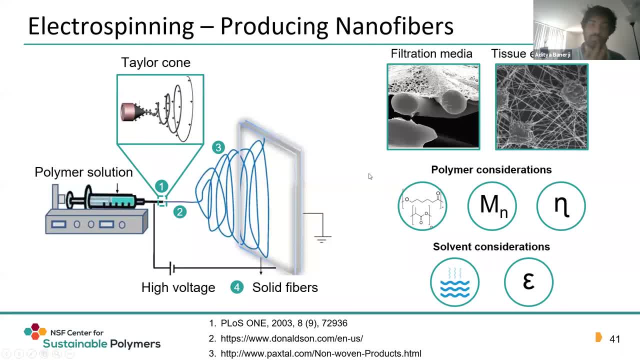 Some of the typical polymer considerations that should be considered taken into consideration in this particular method include the molecular weight of the polymers that are used, the viscosity as well and, more importantly, the dielectric constant of the solvent being used, since electric field is such an important part of this particular process. 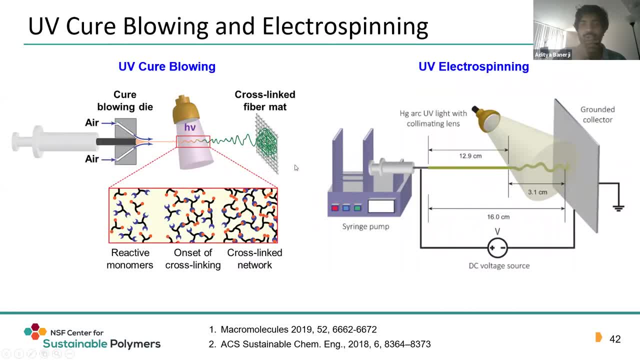 So, moving on, the current research in our group has focused on modifying these melt-blowing and electrospinning methods for what we call UV cure-blowing and UV electrospinning. So what sets these apart from the conventional processes is that, instead of a polymer melt or a polymer solution, 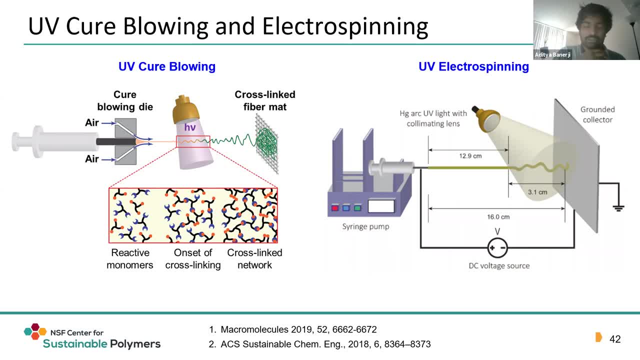 we use a monomer mixture, a reactive monomer mixture, for example, comprising of thiol-acrylate monomers or thiol-allyl ether or other thiol-in monomers that are extruded through a die, which are then drawn by air jets or electric field. 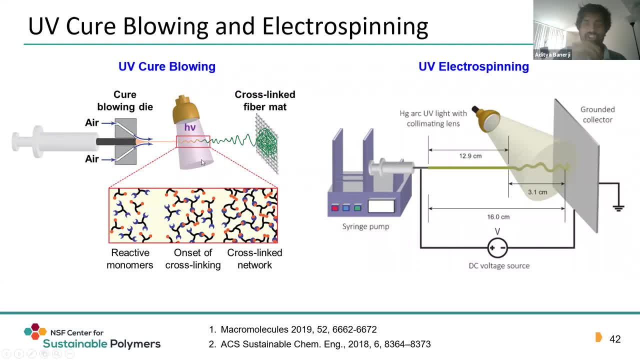 in both the cases, And while in flight, upon shining UV light on them, there's a rapid cross-linking that occurs, which leads to formation of a cross-link network within the fiber mat which is collected. So this also gives an additional benefit that you can get a cross-linked fiber mat at the end of this particular process. 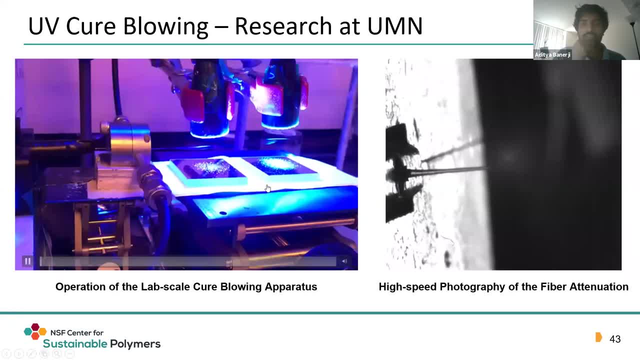 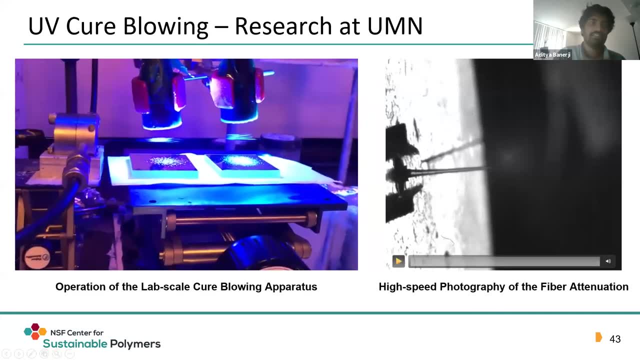 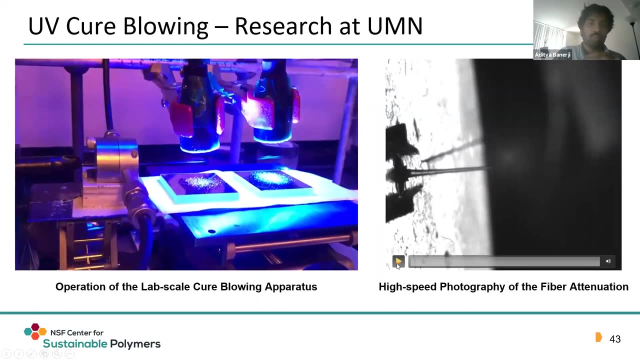 In the next slide I would just show a couple of videos which shows the UV cure-blowing setup that we have in the environment in action, in which you can see that through the syringe on the left the reactive monomers are extruded through the die and during flight upon shining UV light. 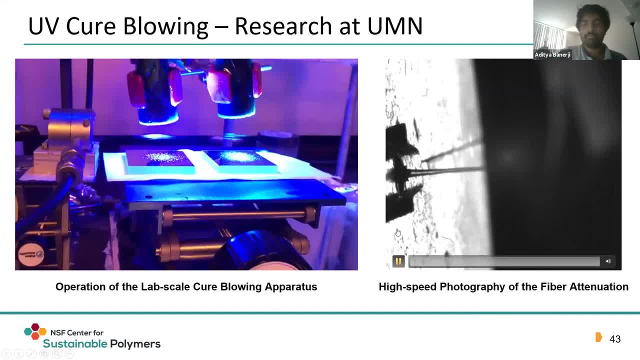 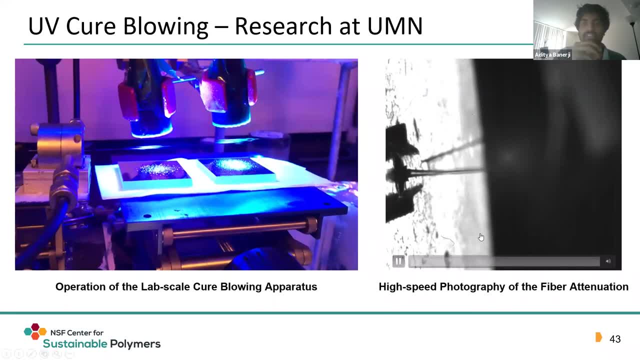 they cross-link, which is collected downstream, While the video on the right basically is a high-speed photography of the fiber attenuation process that is happening, in which high-speed air is impinging on it from the top and bottom slits, And in the video on the right you can see that the fiber slits lead to progressive thinning of the fiber jets as well. 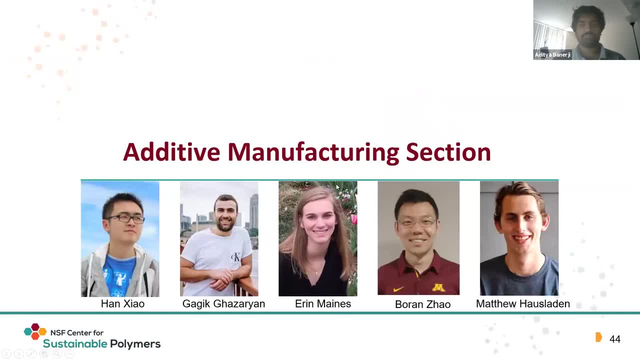 Thank you. Can everybody hear me? well, Yes, we can hear you. You can go ahead. Hello, my name is Boran Zhao. I'm currently a postdoc from Professor Allison's group And in this last section of today's presentation I will shine some light on additive manufacturing, or 3D printing. 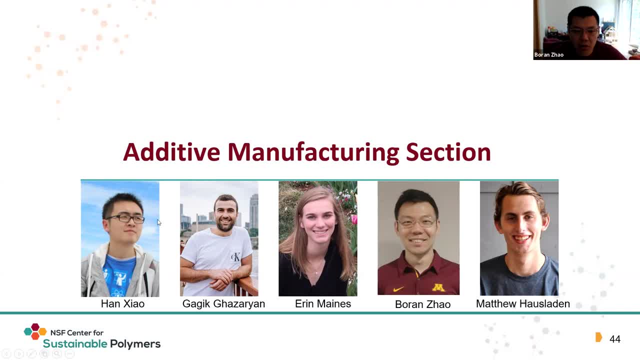 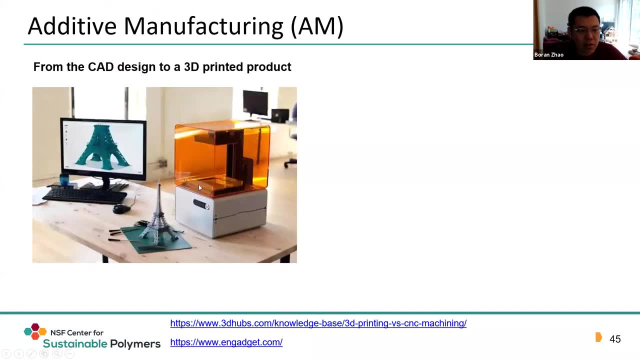 Before I go on that, I would like to thank my colleagues listed here for their help in putting together this section. So the essence of additive manufacturing, or 3D printing, is to translate virtual 3D models from a computer into physical objects. So, as compared to traditional way of material processing, 3D printing doesn't require extensive machining or molding. 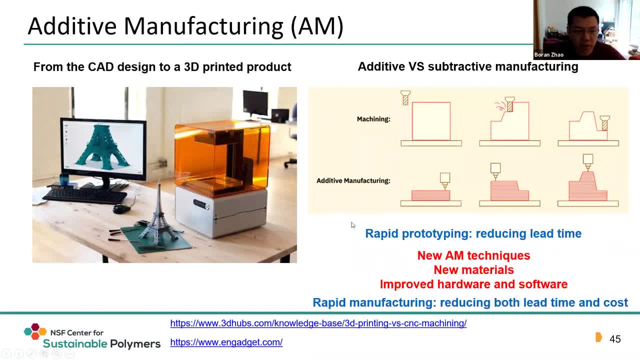 So oftentimes. 3D printing will greatly reduce the lead time in industry And as new 3D printing techniques, new material coming out each year and with improved hardware and software, we will see this trend of transform from rapid prototyping to rapid manufacturing. 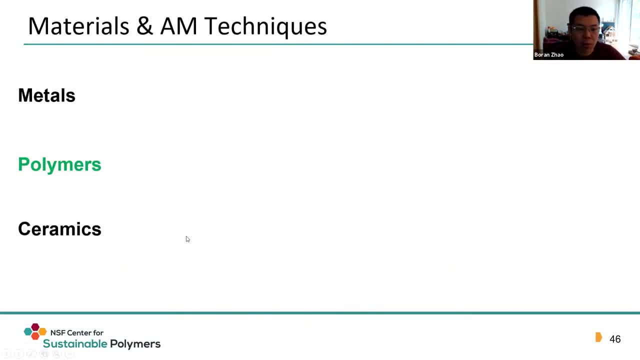 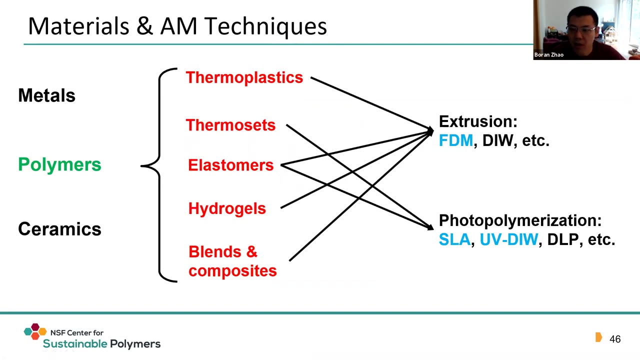 So, among the 3D printing materials, polymeric material definitely plays an essential role And, depending on what type of polymer you are interested in, there are ways of 3D printing method that can process that. Today, I will focus mainly on three most widely used 3D printing techniques. 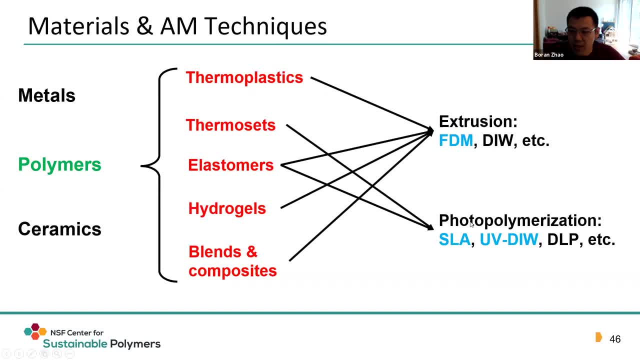 The first one is extrusion-based FDM. The second and the third are photopolymerization-based. They are SLA and UVDIW. In the next slides I will explain what they are, how they work and I'll give an example for each of them. 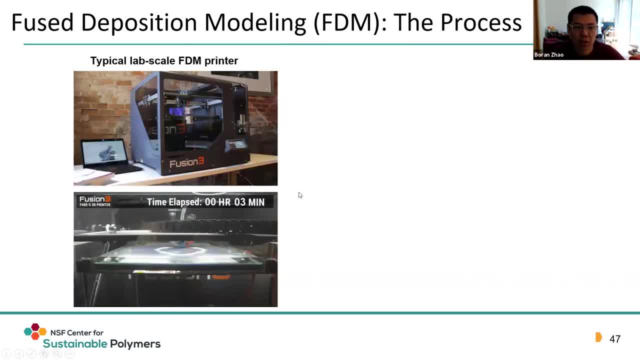 So the first technique I'm going to talk about is called Fused Deposition Modeling. So the picture on the top shows the typical life scale, the size of life scale FDM printer, And the video shown on the bottom shows a typical process of the printing. 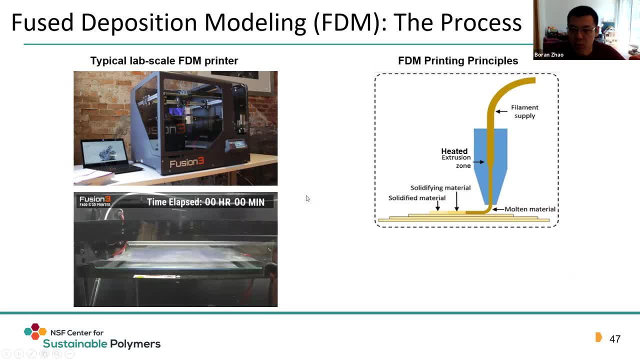 The principles behind FDM printing is pretty straightforward. So we fit in our filament and the filaments get melted, extruded and depotted on the building platform. Here we listed some of the key parameters and dimensions- timescale related to FDM printing. 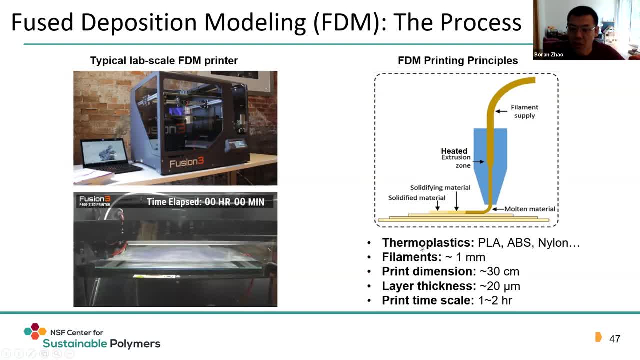 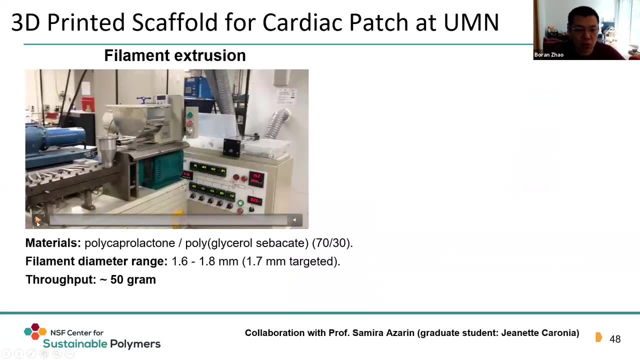 And one thing I want to point out that although there are a lot of thermoplastics, commercially available filaments we can choose from, for example, the PRA, ABS or nylon, you can also make your own filament And in the next slides I'm going to give an example of making customized filament at UMN. 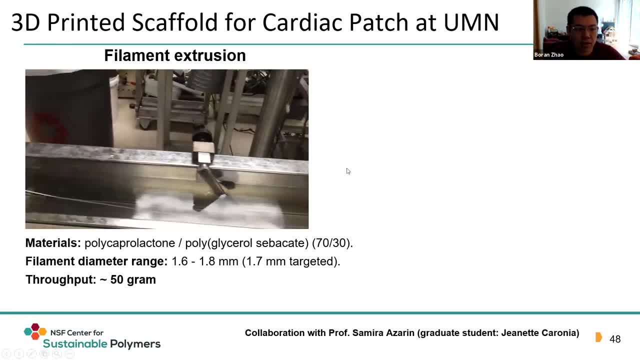 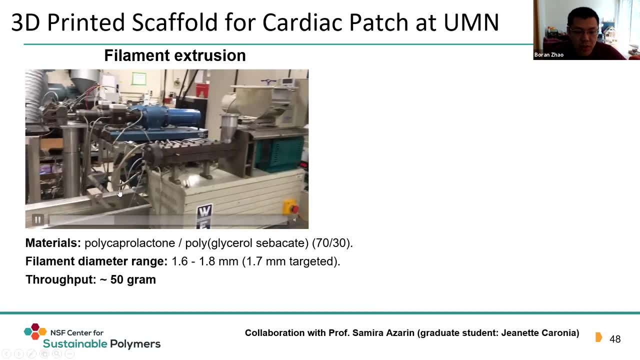 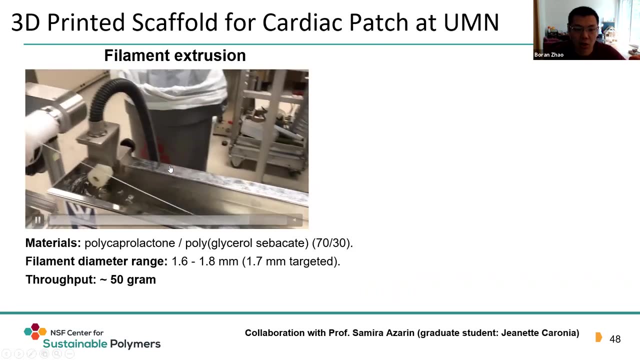 The goal here is to 3D print a scaffold as a cardiatic patch using FDM And shown in the video here. we use the twin screw extruder to make the filament. This is the same, exactly the same extruder that my colleague Charlie talked about before. 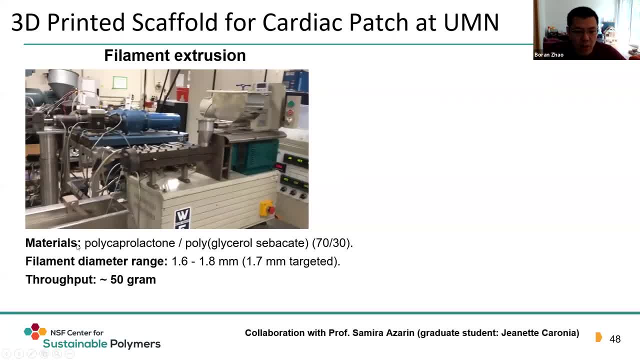 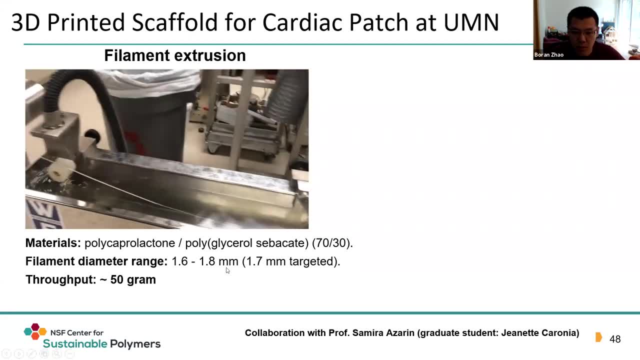 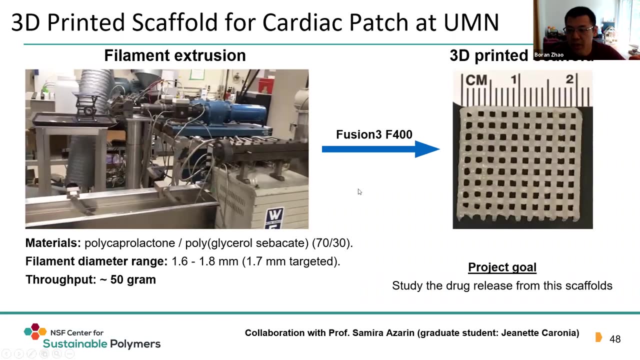 This is, as you can see, like we can, this material is a binary polymer blend And we target the filament diameter to be around 1.7 millimeter, which complies with the requirements from the 3D printer. And here, as the picture shown on the right, this is the final product. 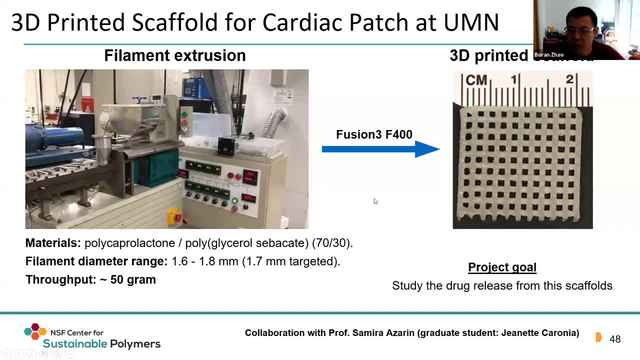 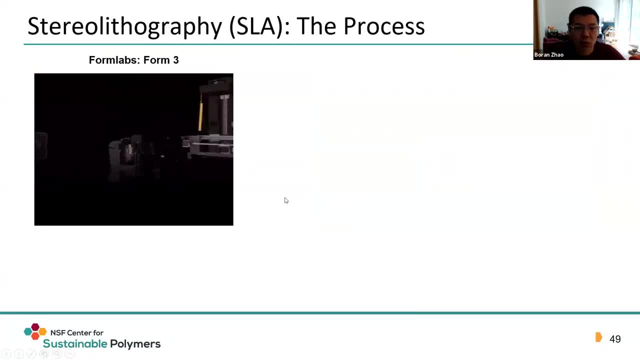 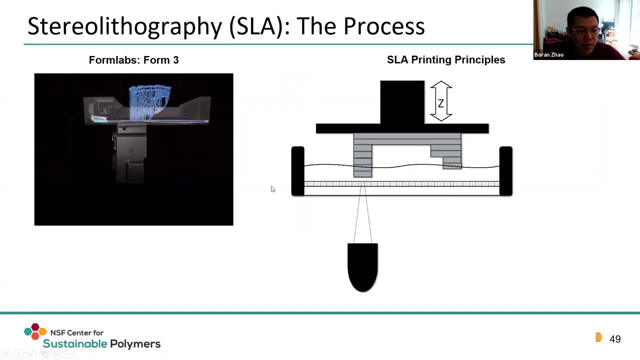 And one thing we want to further develop is to study the drug release from this scaffold. The second technique I want to talk about is stereolithography, or SRA. As the video and picture shows here, the SRA definitely basically converts the liquid resin into a cross-linked part by photopolymerization. 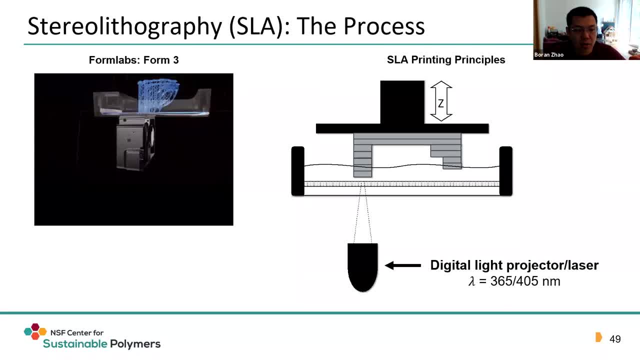 It consists basically three major parts. The first one is the light source. could be either a digital light projector or a single-point laser. The second part is the wet which holds the liquid polymer resins. And third one is the moving build plate. 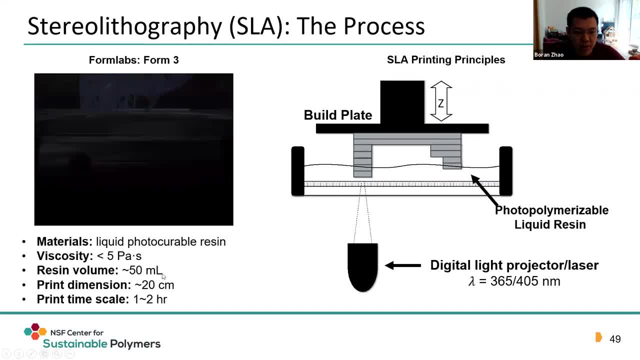 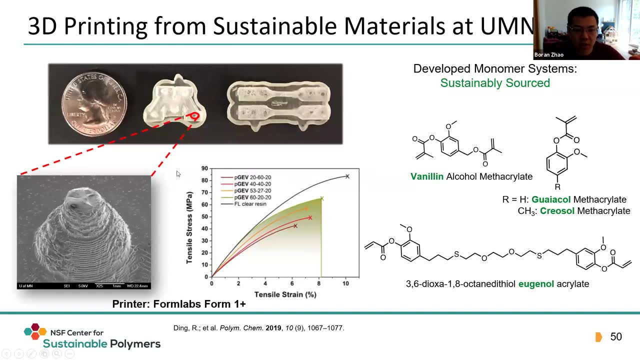 Again. we listed some of the print dimensions here and timescale related to SRA printing And the novel liquid resin for SRA process is definitely a focal point for research And here is an example of the work done at UMN. This is done by Professor Renke's group. 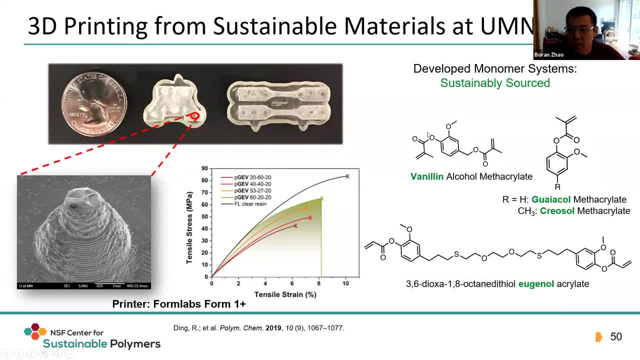 In this work, normal, accurate monomers are developed from phenolic alcohols, And these alcohols are harvested from softwood lignin. They are sustainable And results shown here demonstrate that they can not only generate successful SRA prints. 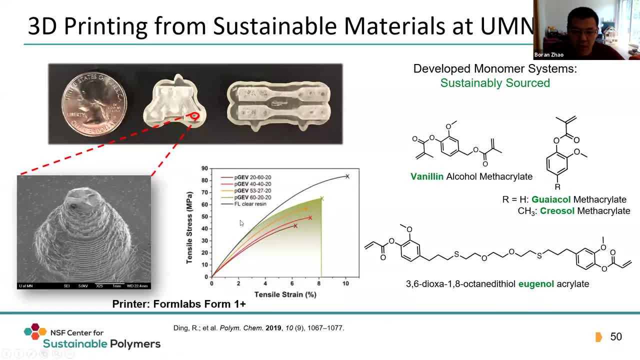 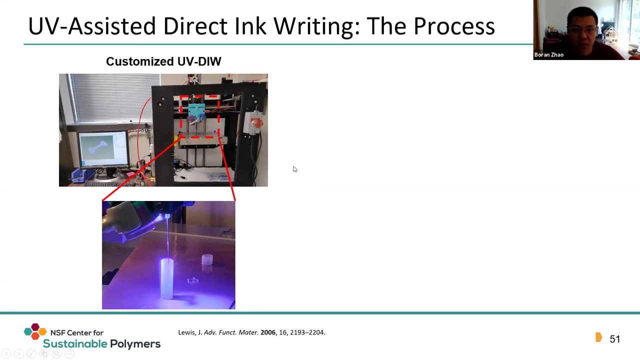 but also the thermal and mechanical properties of these prints are comparable with the commercial SRA resins, for example from FormLab. And moving on to the last technique I'm going to talk about is the UV-assisted direct ink writing. The printing principles looks a lot like a combination of an FDM printer and SRA printer. 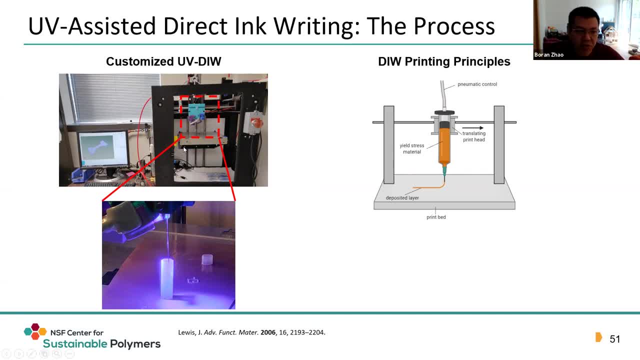 Here is a picture of the printer in Professor Francis' lab. It is converted actually from an FDM printer and we added a UV light attachment. So the liquid resin was extruded to the build plate and it got solidified either continuously or sequentially. 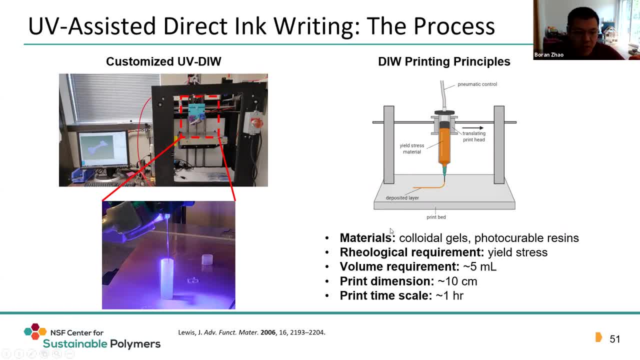 So the resin needs to have a certain yield stress to prevent the resin running away after deposition. And actually the materials are quite flexible. We can use colloidal suspensions, We can use photocurable resins that can be converted from the SRA resin. 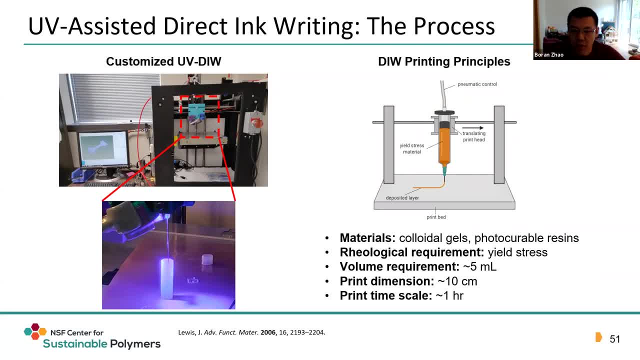 And there are plenty of ways of converting a conventional SRA resin to a DIW resin, For example adding a rheological multilayer. And also, I want to point out, in the lab scale we don't need quite a lot of materials. 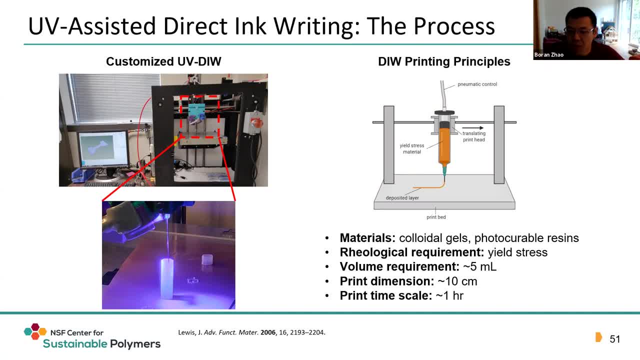 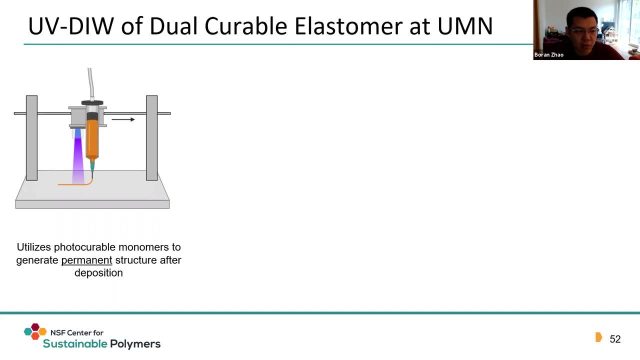 Usually we can generate a print using less than five milliliters, And the printing dimensions could be as large as 10 centimeters and could be finished within an hour. Here I'm giving you an example of the work done at UMN. So from Professor Allison and Professor Francis' group. 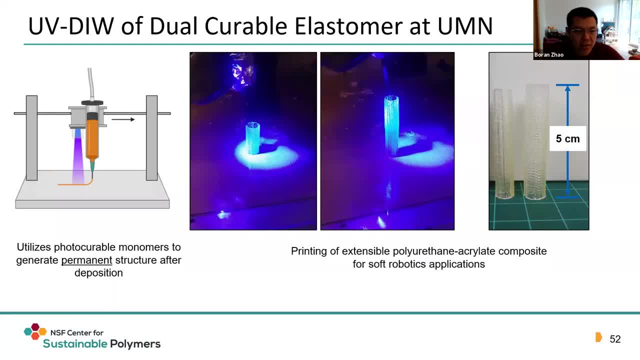 we developed a dual curable resin from acrylate and polyurethane, So the green body is solidified by UV curing the acrylate component and the polyurethane component is cured in a thermal heating process afterwards. As shown here, we can generate fairly high aspect ratio of these elastomers. 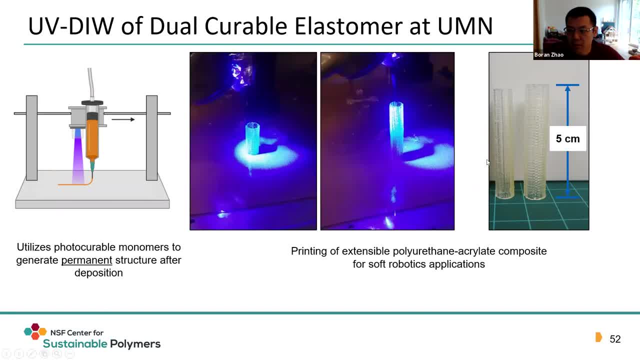 And based on different components of acrylate and polyurethane. this print could be in a rigid body or could be as extensible as an elastomer, And these are perfectly suitable for soft robotic applications. And that's the end of my section and I will turn it over to Professor Allison. 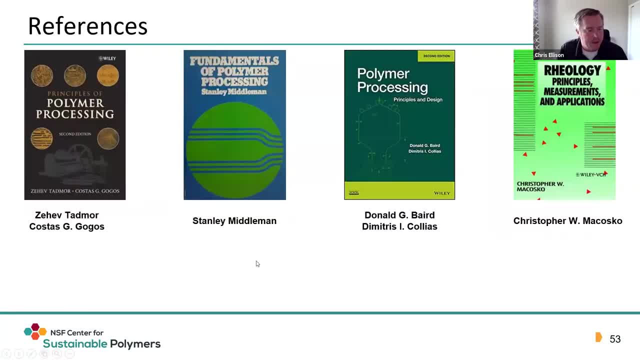 Okay, Maybe before I wrap up here, I just want to make a quick comment. Maybe some of you have seen Chris McCosko and myself chatting back and forth, but don't let the scale of some of the instruments scare you. Some of them indicate 500 grams is sort of the scale you operate at. 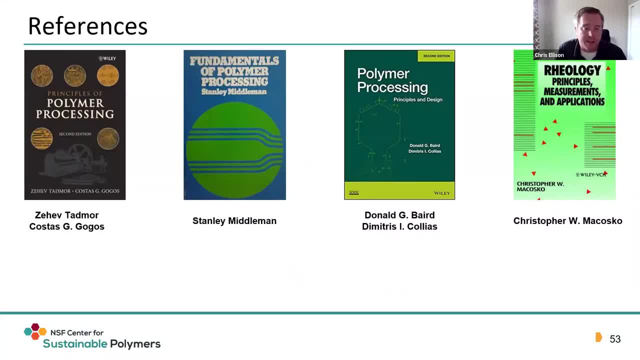 but there are really clever ways to inject a plug of, let's say, active material, material that may have some special chemistry incorporated into it or some other special properties, that you can inject a 50-gram plug in the continuous process to make a run of a sample that could be of interest to your research. 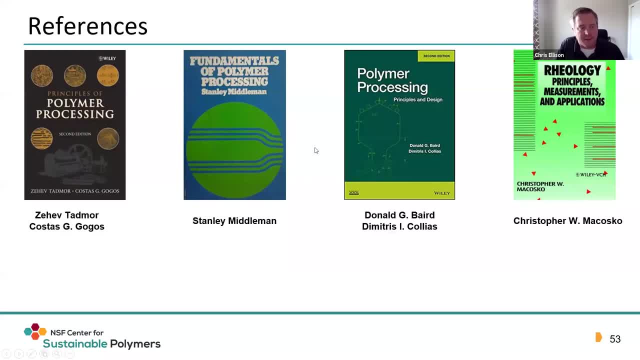 So don't think that you need 500 grams exclusively. There are ways to get away with smaller amounts. To conclude a little bit, I just want to point out that there's a lot of really nice references that you might take a look at as you start to think about processing. 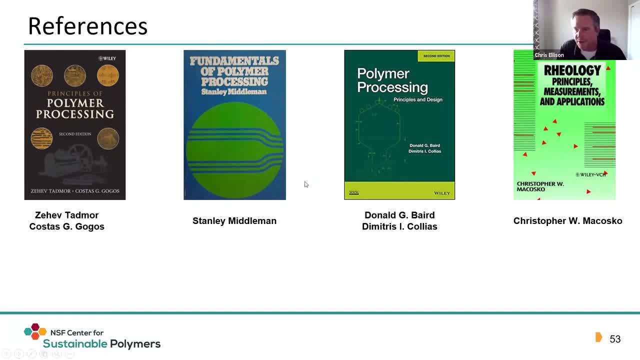 and these are just a few of them here. Obviously there's many others, but I like these versions because they both broadly cover different processing operations, but also they really bring out the focus of the material and how it might interact or change its viscosity, et cetera, in different types of processes. 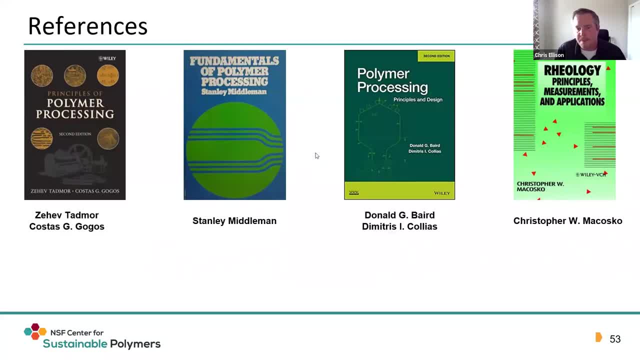 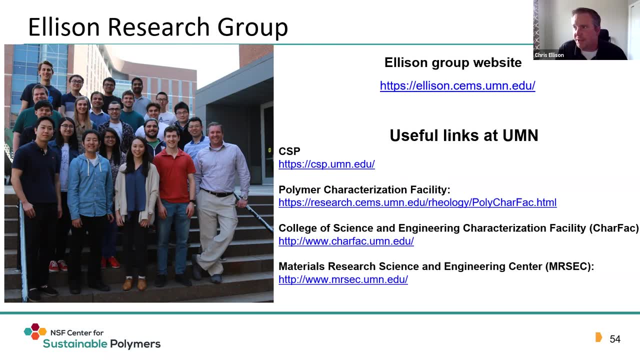 So take a look at these if you have interest in reading further. And finally, I want to thank again all of the members of the Ellison group that helped put this together. This was a non-trivial exercise to put all these slides together and we got a lot of nice feedback from Chris McCosko. 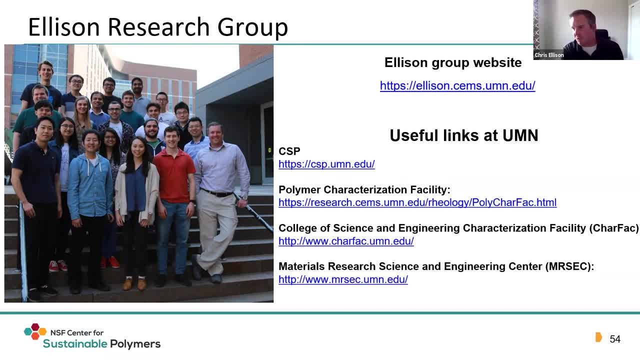 and I thank him again for his help. And this is the group. not too long ago, Many of the people have contributed that you see here and some of them have contributed. They've been presenters today. We'd love to collaborate with any of you.